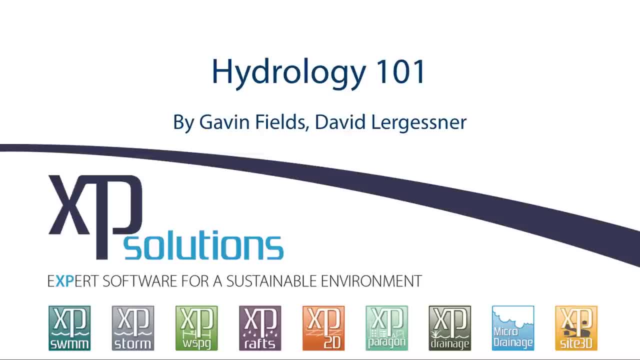 as well as being a significant contributor to the Cambridge series Geography for the Australian Curriculum, David's passionate interest is sharing how a knowledge of geography is fundamental in seeking solutions to people and environmental management issues locally and around the world. So today we'll run through first of all, what is geography and what is geomorphology. 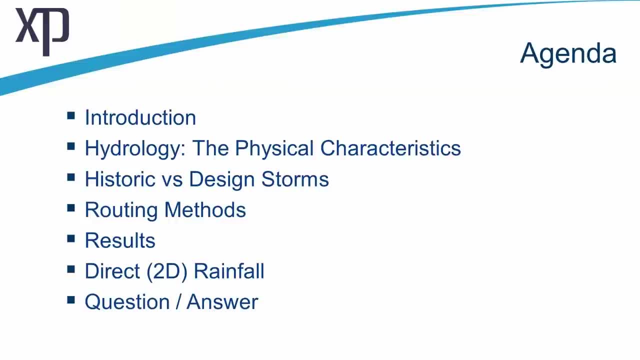 So today we'll run through first of all what is geography and what is geomorphology. First a brief introduction, then discuss the physical characteristics of hydrology, look at various different rainfall methods, routing methods, talk about how you present hydrological results and how hydrology affects 2D methods as well, followed by our question. 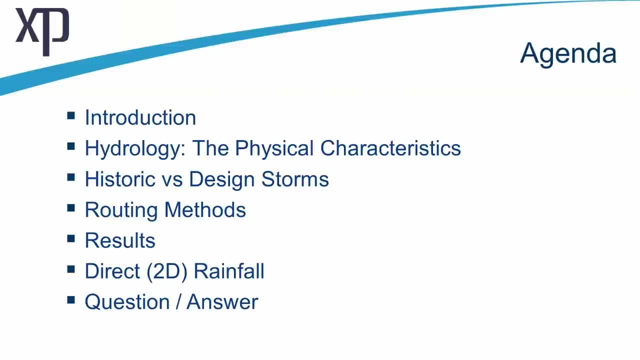 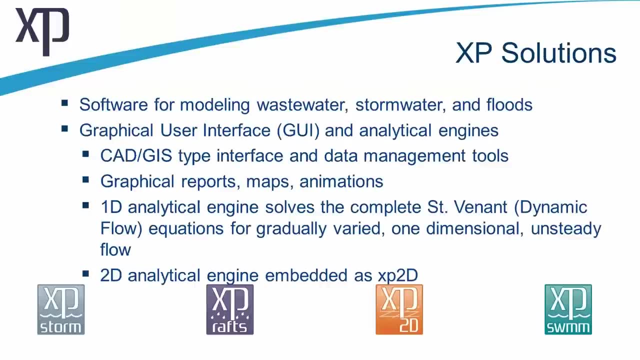 and answer session. For those of you who don't know, XP Solutions, we're a software company for modelling wastewater, stormwater and flooding. We have an advanced graphical user interface and analytical engines. The software produces CAD and GIS type interfaces and data management tools, as well as graphical reports, maps and animations. We have hydrological 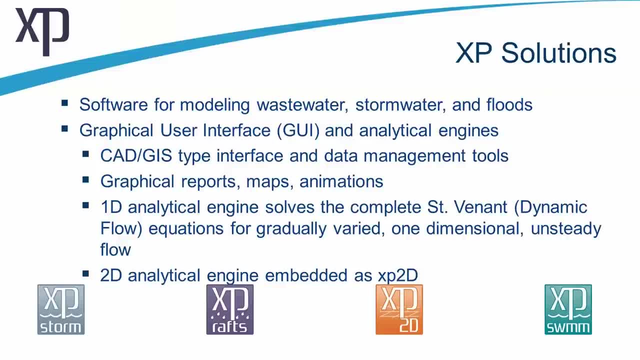 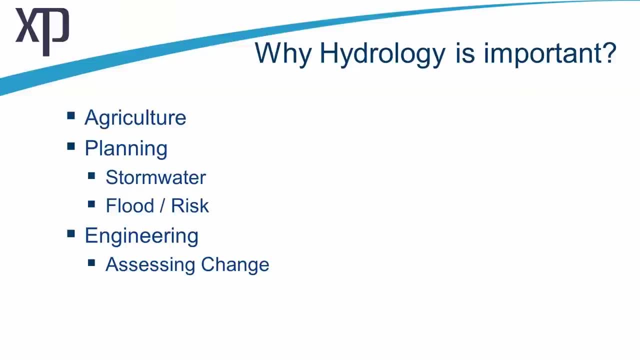 methods built into the software: 1D analytical engines and252D analytical engines embedded as XP2D. So why is this important? Well, obviously there's a wide range of people that use hydrological data In agriculture. it's very important to know what happens when we receive rainfall. 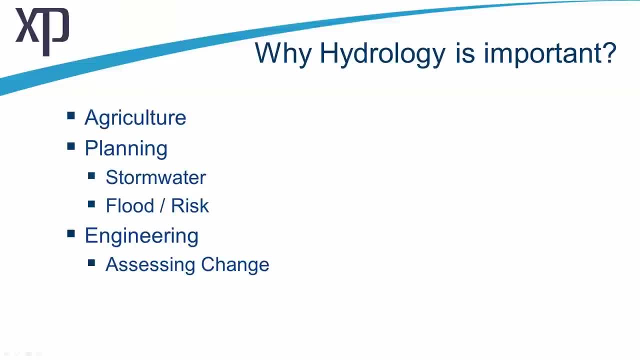 onto the land and how that runs off and how we manage that water. When we're planning towns and cities, we need to know where the stormwater will go and where the risk of flooding is in order to make sensible decisions about development And in other areas of engineering. 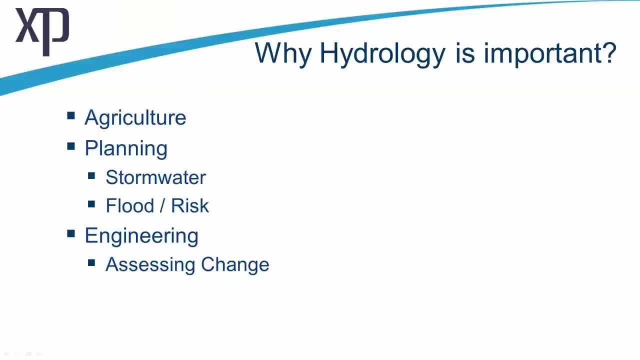 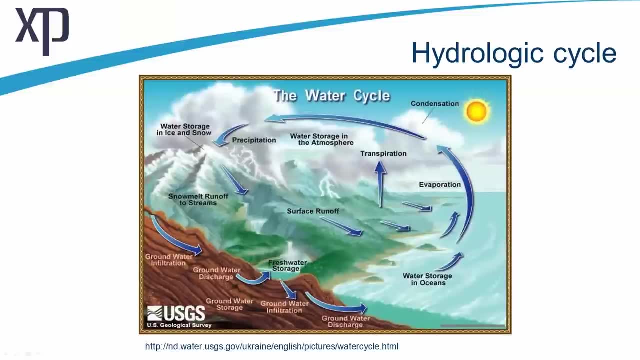 we need to assess the change, and you'll hear more about that from our speakers during today. So first I'd like to welcome David. Thanks very much, Jessica. it's great to be here today. Let's kick off at the start of the thing, and that's the hydrologic cycle, Probably. 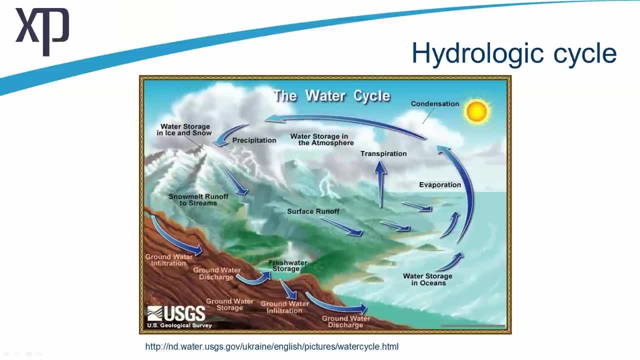 most of us are familiar with this sort of diagram. we've got up here now. We get the evaporation off the ocean, we get condensation into clouds. clouds move inland, they're pushed up by the mountains. rain falls rain and precipitation in various different forms of 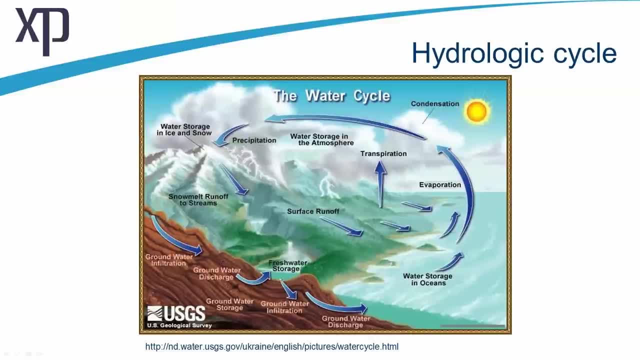 ice and snow, sorry snow, sleet, rain, And of course that's the hydrological cycle. Of course, this eventually runs off down slopes and either into streams, into storages, and finds its way back to the ocean where the cycle begins again. 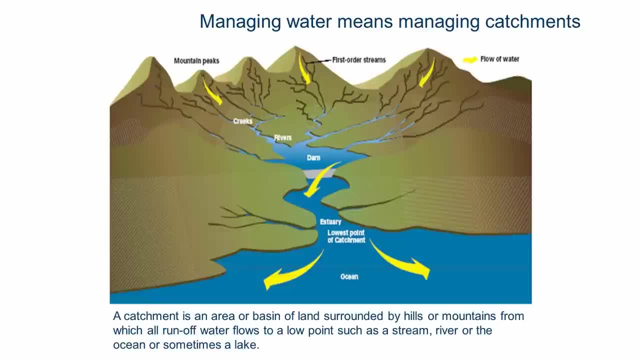 And most of the things that we're looking at, of course, in terms of managing water and looking at hydrology, is looking at catchments on the earth's surface. There are various sizes of catchments on the earth's surface and the important thing is that a catchment 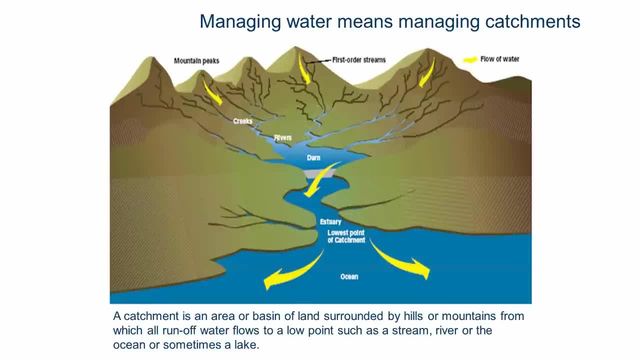 is an area which collects all the runoff from a particular area, directs it to a low point such as a stream or a river, and then it's collected, and then it's collected into a stream, river and or lake sometimes, and sometimes it'll go to the ocean, but if it's 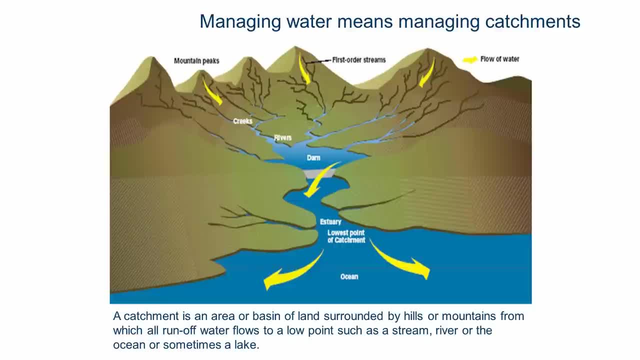 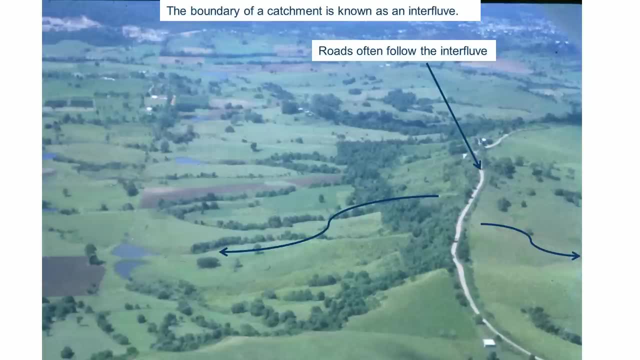 an internal place like Australia, a lot of it might evaporate internally. Right. the boundary of a catchment is known as an interflueve French word meaning between rivers, and in this slide here we've got the actual boundary of the catchment: the interflueve. 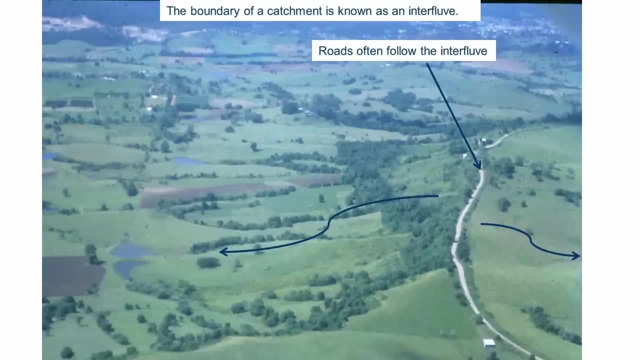 is actually followed by the road and roads often do follow those sort of areas. You can see on the left hand side, the water, the stream, the river. On the right hand side, the water's running into one catchment area. on the right hand, 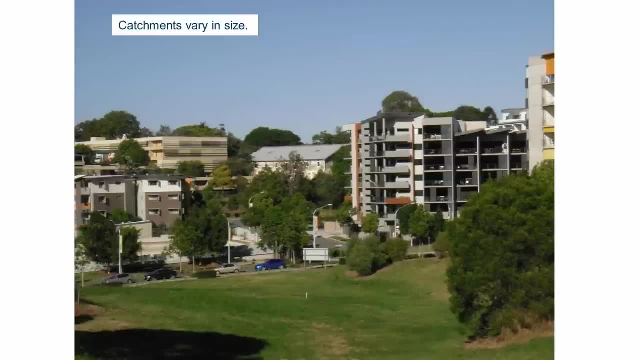 side the water's running into an entirely different catchment area. Okay, as I said, catchments vary in size. This is one of the smallest I've seen- fascinating little one here in Kelvin Grove in Brisbane and I was just lucky I got that photograph. 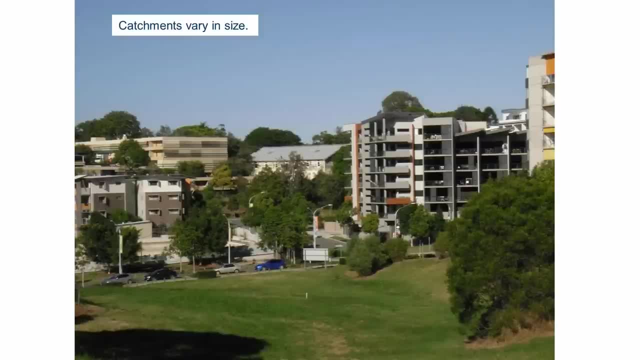 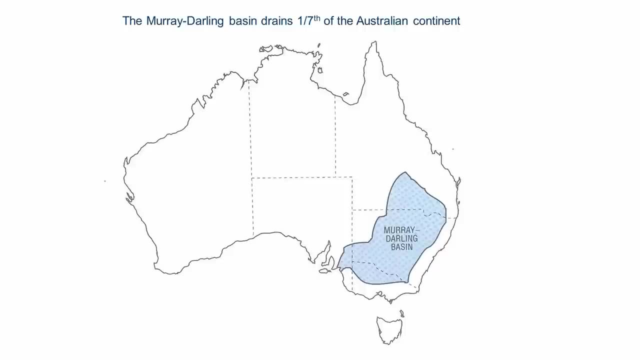 a couple of years ago, because there's now a 17 storey building built on that particular site. Much larger sort of catchments, of course. the Murray-Darling Basin is the largest one in Australia. It drains one seventh of the Australian continent and starts up in Queensland, New South Wales. 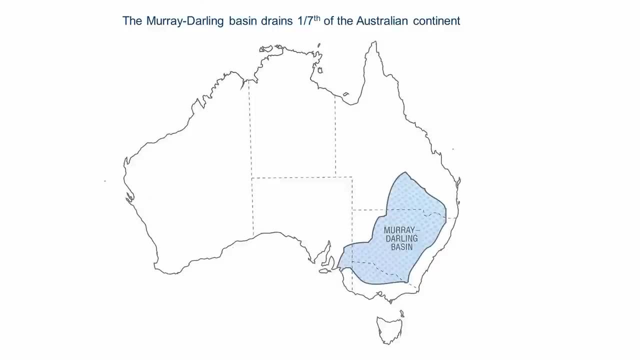 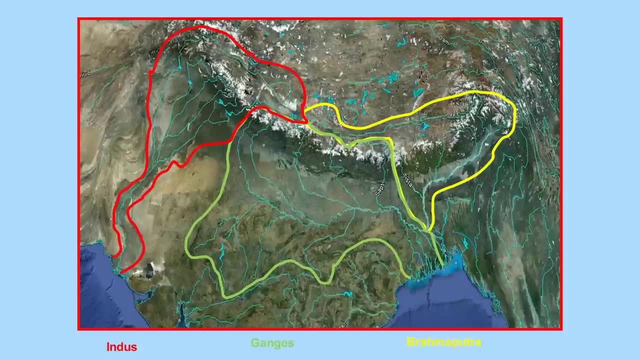 Victoria flows down to South Australia and also includes part of the Australian Capital Territory as well. Just a slightly different thing for those people here, because we've got people from all around the world have joined us today, and I think that's great. In the Indian subcontinent, three very large catchment areas there, the Indus River rising- 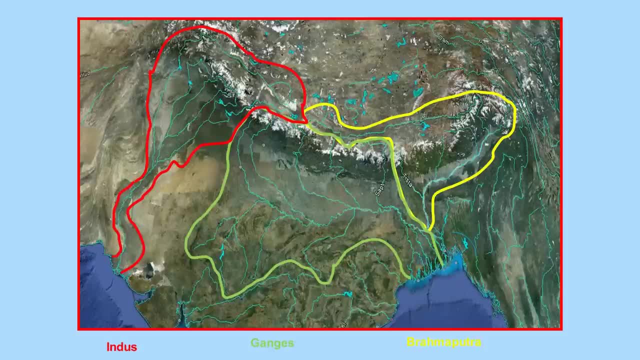 of course, in the Himalayan mountains And flowing down towards the southwest there, circling around the western side of the Thar Desert, The northern side of the Himalayan mountains, we have the Brahmaputra River flows parallel to the Himalayan ranges there for quite a while before it cuts through the ranges and 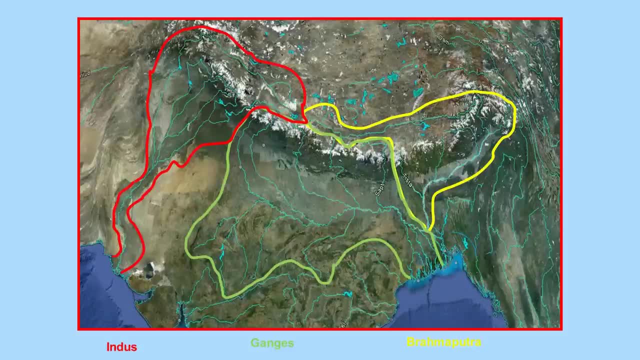 makes its way down, where it actually flows into the Ganges, which, of course, is the largest catchment that we've got in this particular area there, And you can see the rivers coming out of the Himalayan mountains there, some of them running off the Deccan Plateau to the south and finding their way into the Bay of Bengal. 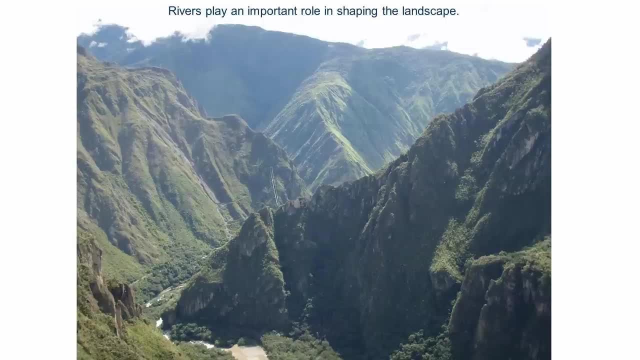 Rivers play an important role in shaping the landscape around us. This particular picture here comes from South America. The mountains there are being pushed up by lots of action in terms of tectonic plates crashing into each other and grinding against each other, pushing these mountains up. 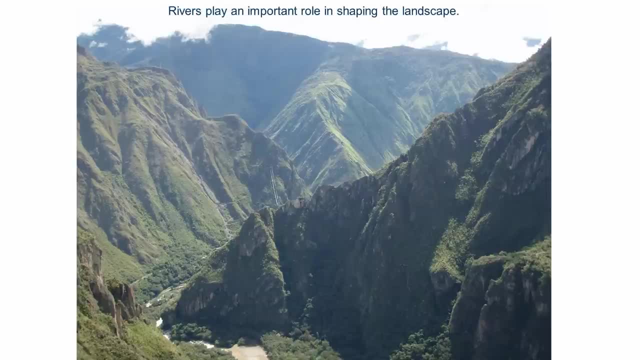 And, of course, once they're pushed up, of course the rains start to pour down on them And you can see the rivers coming out of the Deccan Plateau to the south and finding their way into the Bay of Bengal. This particular picture here comes from South America. The mountains there are being pushed up by lots of action in terms of tectonic plates crashing into each other and grinding against each other, pushing these mountains up And, of course, once they're pushed up, of course the rains start to pour down on them and start 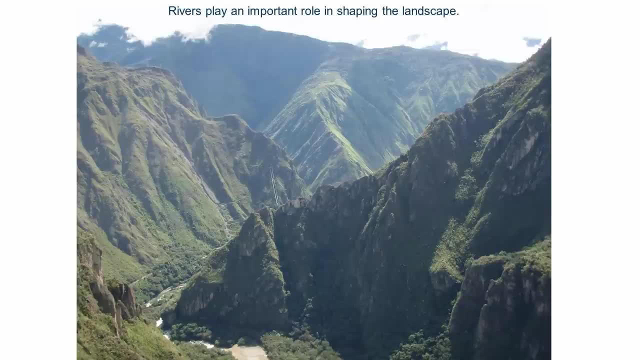 to erode away the particular land surface And in this particular instance we've got these very steep V-shaped valleys in the headwaters of that particular catchment area. It's only very small headwaters because it's very soon that the actual Amazon River flows. 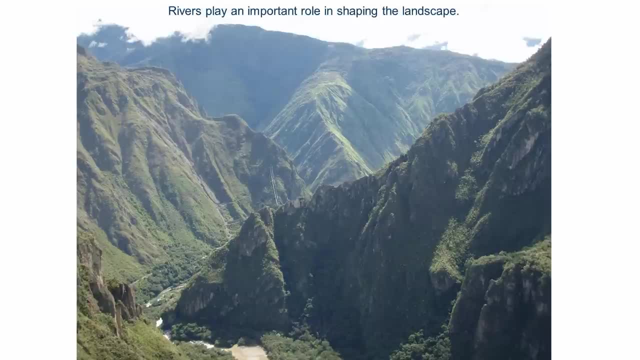 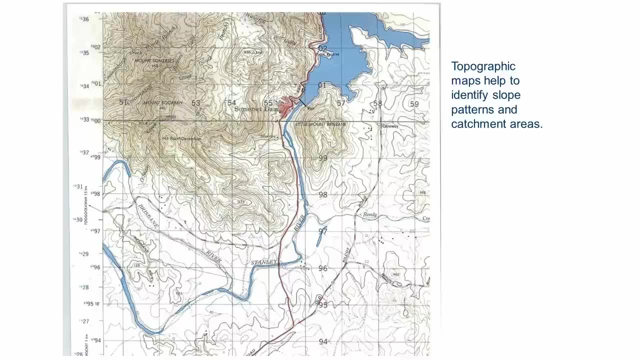 out into that large plain, which, of course, heads off to the Atlantic Ocean thousands of kilometres away. Topographic maps are useful in terms of identifying rivers. Topographic maps are useful in terms of identifying rivers. Topographic maps are useful in terms of identifying rivers. 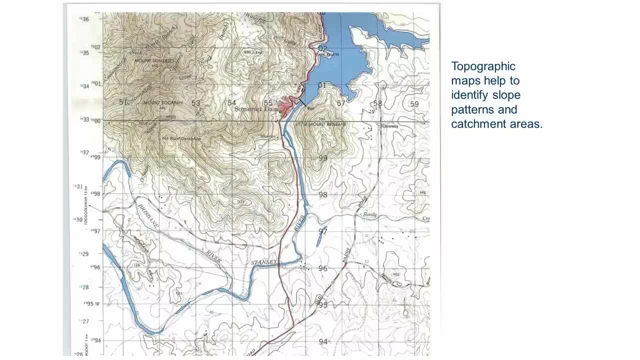 Where catchments are. this particular one is an extract from the Brisbane River area, and you can see sometimes how difficult it is to interpret these maps. You can see in the northern, north-western part of this particular map there's quite some rugged terrain there, quite a lot of ridges, narrow valleys, and so it's quite 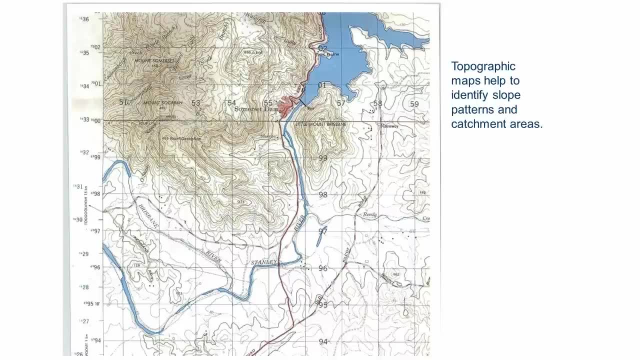 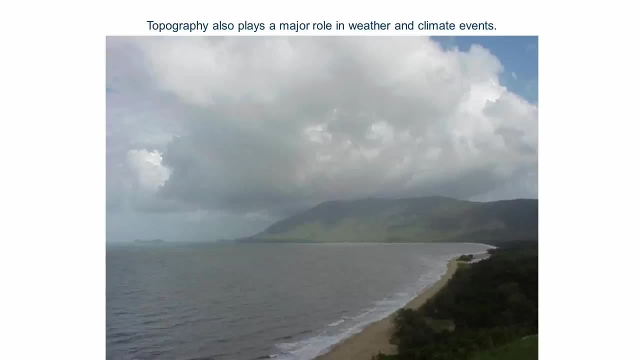 interesting to try and actually work out where the catchment boundary is between sub-catchments of the main catchment of the Brisbane River in this area. Quite complicated on the north-eastern side, not so difficult on the south-eastern side, North Queensland, where we have the ranges come down quite close to the coast in this. 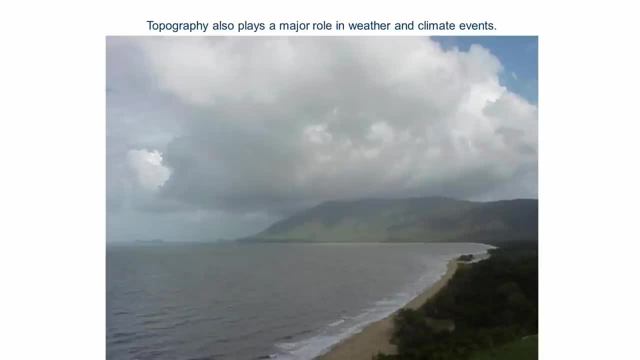 particular area. When the winds blow off the ocean, as they frequently do, they are pushed up against these mountains. here they rise against the mountains and as they rise, of course the air cools. Because the air cools, it can't hold so much moisture. 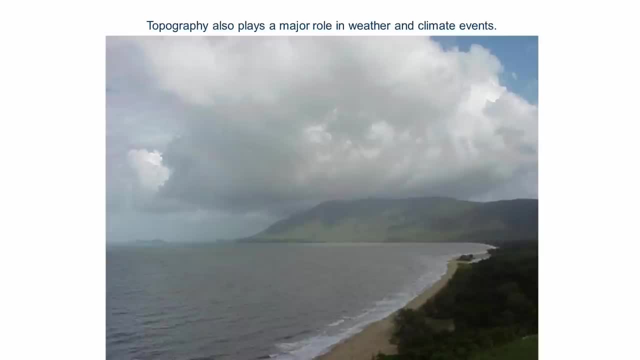 And so the moisture condenses out to form clouds. Probably in many instances those clouds will evaporate later on in the day. Sometimes they'll build enough so that we get quite a significant amount of rainfall in that particular area. That happens in a number of parts of the world which we'll see in a couple of secs. 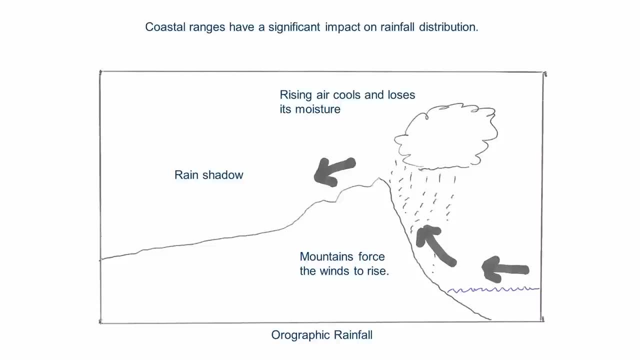 Okay, there's the diagram to represent what we've just looked at. We've got the wind coming in off the ocean, being forced to rise by the mountains in this area, Clouds forming Rainfalls, But the interesting thing is is that the rain falls on the ocean side of the mountain. 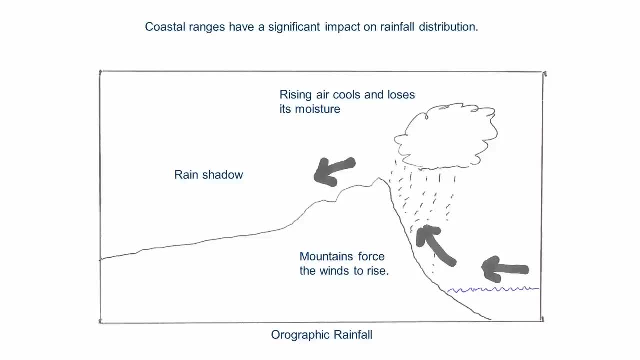 Once the winds get over the mountains, we tend to have very little moisture in them, And so we get what's known as a rain shadow in that particular area. That means we've got quite different hydrologic regimes in that area, Quite different runoff and types of runoff in those sorts of areas. 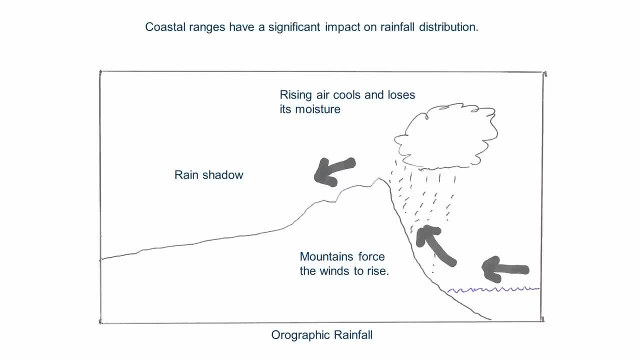 There's quite steep fast-flowing rivers on the eastern side of that mountain. Okay, There's quite steep fast-flowing rivers on the eastern side of that diagram. Quite slow-flowing rivers on the western side. Thanks, Great dividing range. 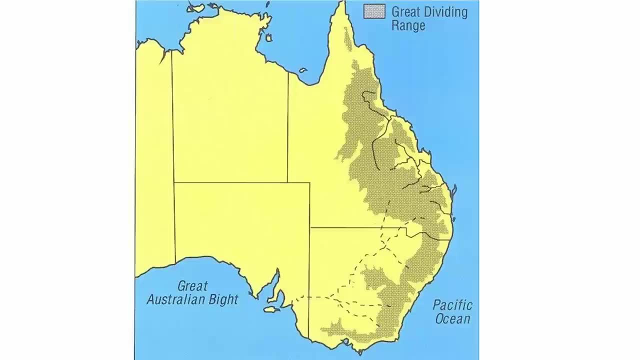 It comes down right down the east coast of Australia, And so we have that effect and it's very, very pronounced in the northern part of Australia, Not so much further down the coast here, but we do get a separation of the rainfall patterns. 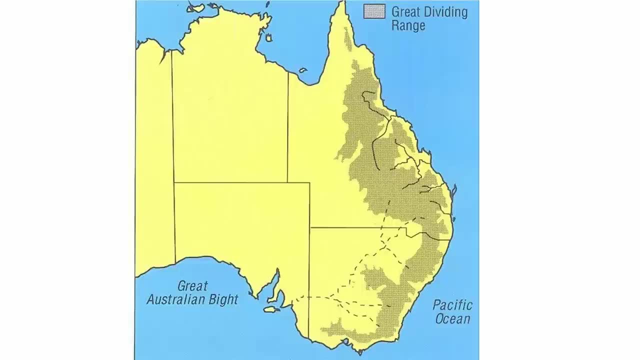 with the rain on the eastern coast areas and the much drier inland areas And the diagram we've got there in front of us. you can see some of those shorter rivers Which flow out of the dividing range in this area And then the much longer rivers which flow down to the South Australian area. there 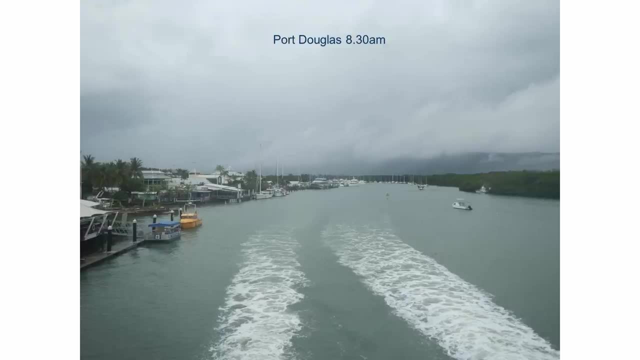 Of course that's the Murray-Darling Basin system there. Thanks, Right, That's just a classic one here. I was on the Barrier Reef a couple of weeks ago, and this photograph just shows exactly what we've been looking at. 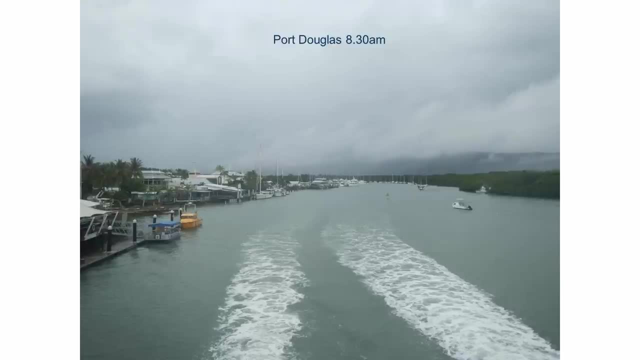 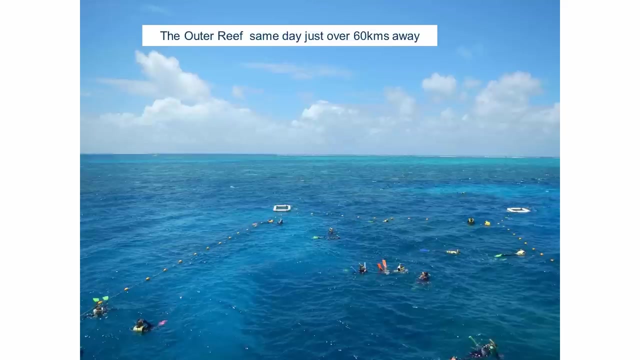 How the mountains here have built the. you know, the clouds have built up against the mountains And when I left Port Douglas that particular day it was quite cloudy and overcast. It had been raining earlier in the morning, But just a couple of minutes later we're out on the outer reef and it's a totally 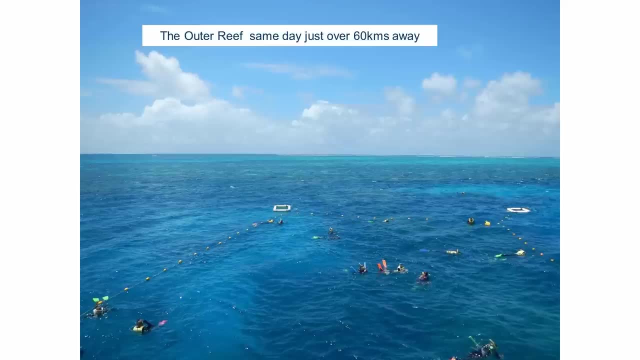 different scene because we don't have the same sort of buildup of clouds in this area. It's just a pity I didn't go the other direction, over the range instead of out of the reef, Because over the range is a town called Mareeba and it prides itself on having about 300 rain-free. 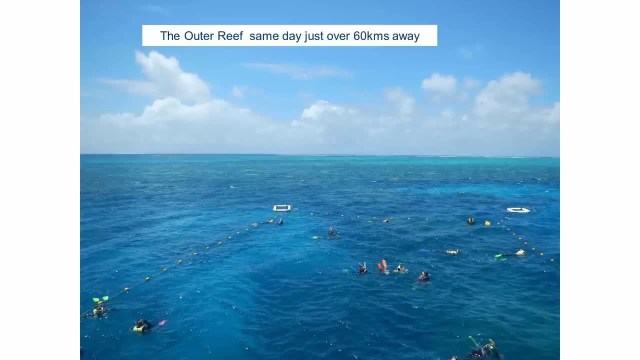 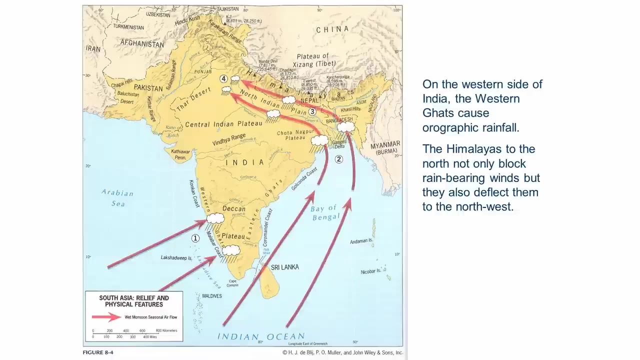 days a year. So it would be interesting to compare Port Douglas and Mareeba, but unfortunately I was going to the reef that day. Right, Looking at other parts of the world where we have the same sort of thing happening. Right, The monsoons in India are a very important weather pattern in that particular part of 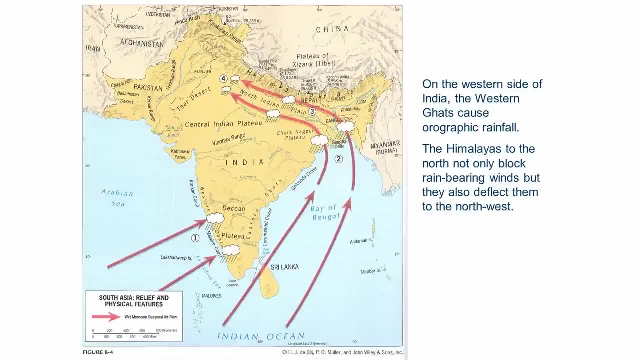 the world. The wind blows in from the Indian Ocean and Arabian Sea in the southwestern there and it sweeps across the Indian area. It's called the Western Ghats there, on the western side of India, And the rain you know they do force. they're only about 2,500 metres high, not very high. 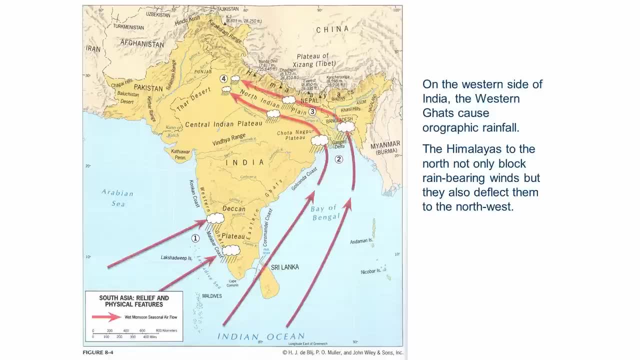 really. but they're high enough to push those clouds up and get the rain falling in that particular part of the area. So you get a drier Deccan plateau. but then, as the winds go out across the Bay of Bengal, they pick up more moisture and of course they bump into that Himalayan range in the 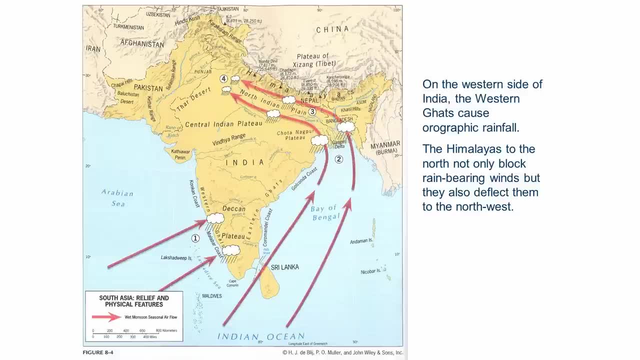 northern part of the area there and that forces the rain-bearing winds off to the northwest. there Lots of the rain falls on the mountainous areas and, of course, lots of the rain falls on that north Indian plain there too, Very important for that particular part of the world. 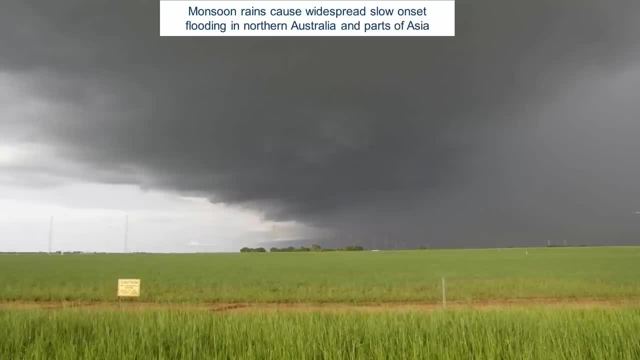 Right, Sorry. Northern Australia also has an interesting pattern in terms of monsoons, because we get a quite virtually a six-month dry period and a six-month wet period. This particular time I was just it's coming back from Kakadu. you can see it's coming. 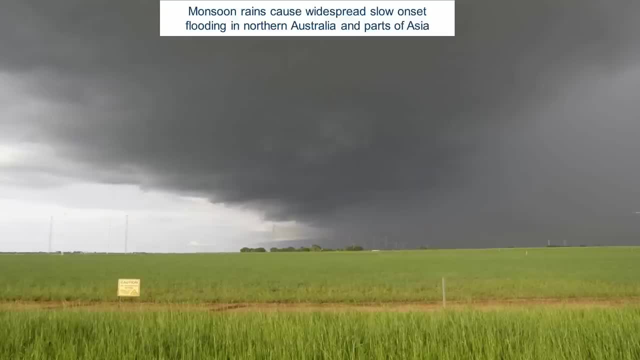 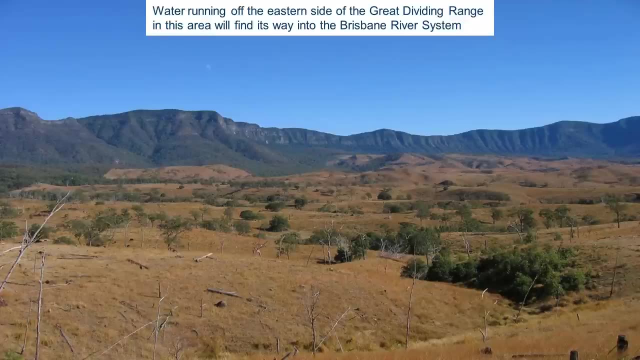 up behind me. It's coming up quite quickly there and there's quite heavy rain falling in that particular area at that time. Right Here we are again looking very clearly at what's the catchment boundary in this particular instance. This is the Inder Fluve here. 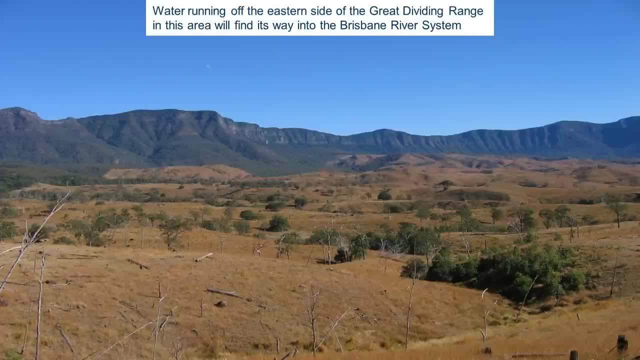 Any rain which falls in this area, in front of me here or in front of the slide you're viewing there, will flow into the Brisbane River and be part of the Brisbane catchment right If it flows. however, if the rain falls on the other side of the mountain, that's the 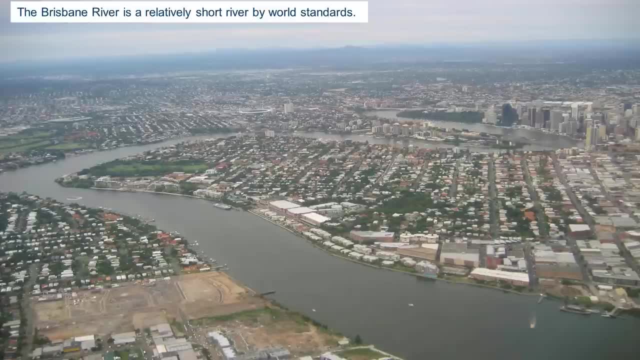 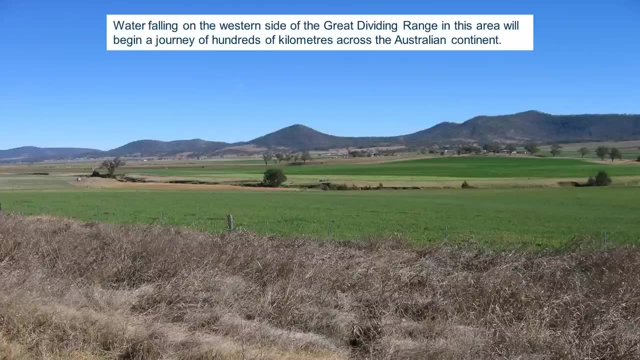 Brisbane River. there It's not a very long river. You can see those mountains in the background there, and if the water falls on the other side of the Great Dividing Range, then it starts a very, very long, slow trip virtually right through the Australian continent, as we've seen in a couple of slides so far until. 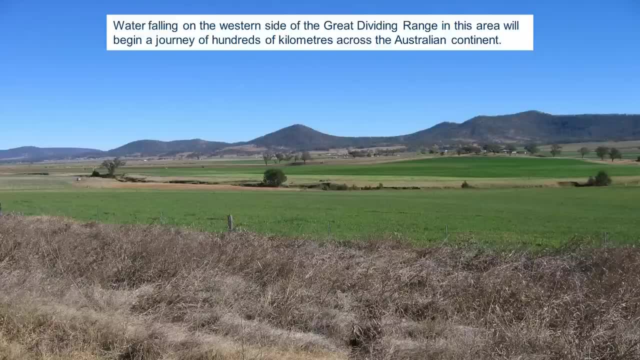 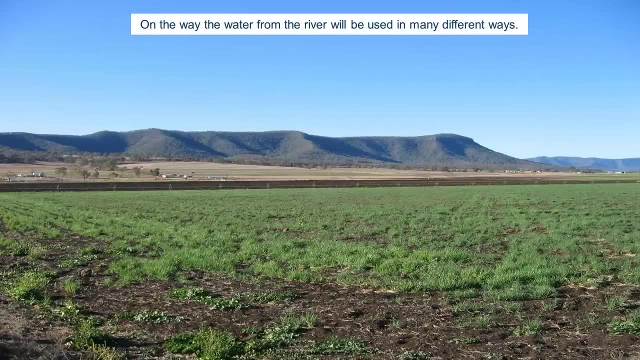 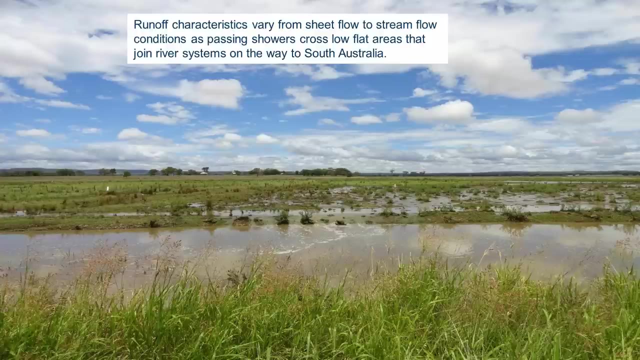 it reaches the ocean. Of course, some of it never reaches the ocean because it's used for agriculture, urbanisation and so on. It's used for irrigation purposes, urban purposes along the way. This was a result of a particular storm that happened as I was going through this area. 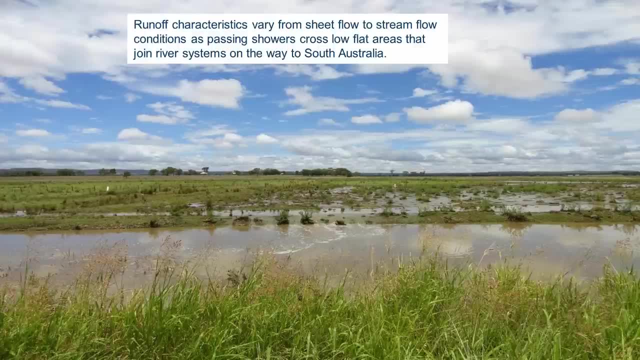 You can see the runoff here from quite a very flat area. It's sheet flow across the surface there until eventually it comes into the drainage channel in the foreground here and, as I said, that water will find its way eventually, some of it to South Australia. 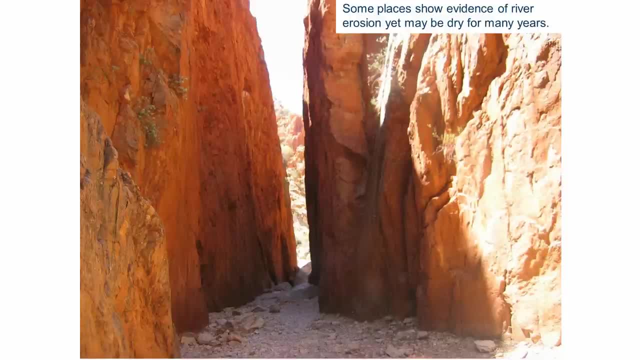 Some places, on the other hand, can be dry for years and years, and years at a time, and then, all of a sudden, we get a lot of rainfall in a very quick period and you have quite quick flows through these particular environments. 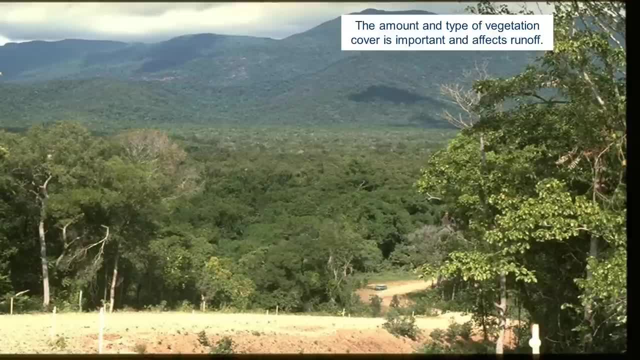 Now we've looked at the rainfall, precipitation and that particular aspect of hydrology. What sort of things now interfere and impact on the amount of runoff which we get in a particular area? This slide we've got here shows quite distinctly the impact of the rainforest in North Queensland. 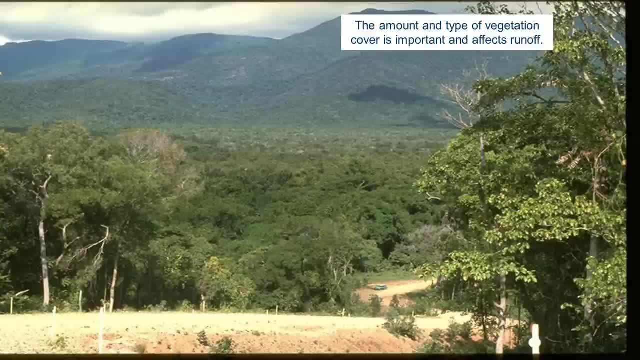 This is a Daintree rainforest. here You can see that, except for the road, in this area the actual vegetation cover is quite complete. And just on that point, one of the key elements as an engineer that we see in this particular photo is a discreet variation between surface roughness, obviously in the form of Manning's. 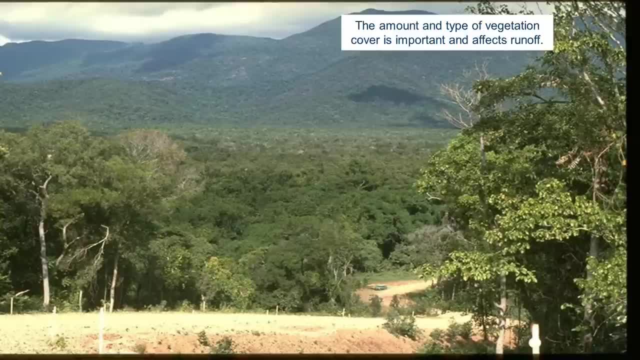 End from an engineering perspective And where we might expect, on the gravel road. it's not. It's not. It's not That that manning's value may be as low as 0.02.. We're reaching up to quite high values as we get up into the upper reaches of that slope. 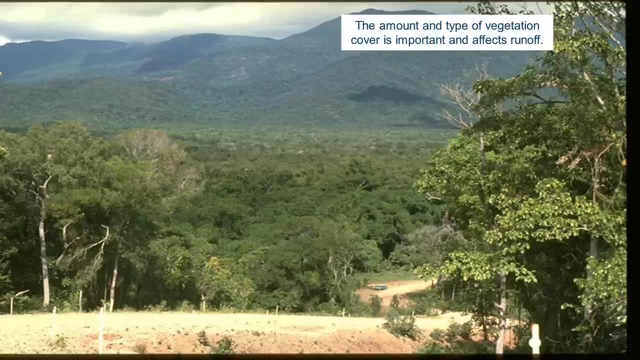 where the manning's value may rise to 0.15 or greater. Thanks, Gav. And the interesting thing here, of course, is that it's such a closed canopy. it makes it very difficult for the rain, when it does fall, to actually get through to the lower. 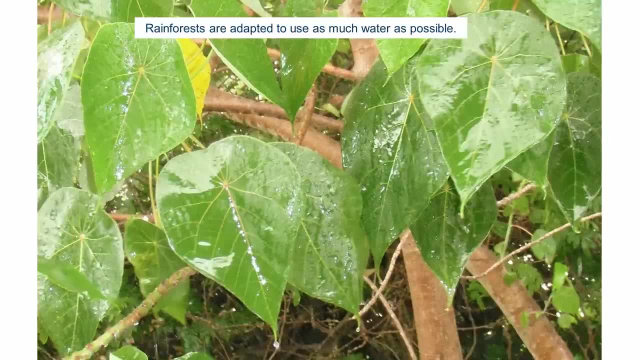 layers. Now the rainforest depends on this water getting through to the lower layers. It's very, very important through to the lower layers, and so they've adapted quite significantly. in terms of the whole canopy acts virtually as a sponge collecting water, and some of that water will evaporate. 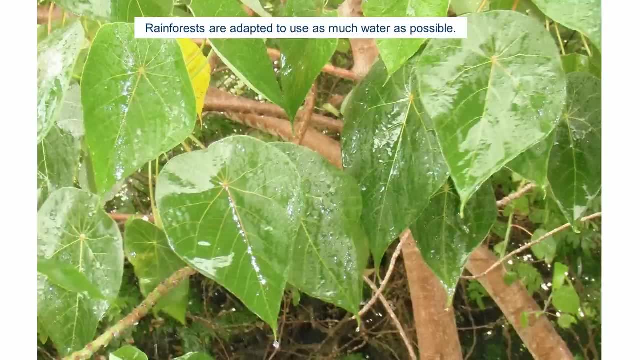 back into the atmosphere. but if the plants- and many of the plants in rainforest areas- are specially adapted and they have leaves- like this particular Macaranga plant which I have in front of us here, has a large leaf to catch a lot of water, then it has a very 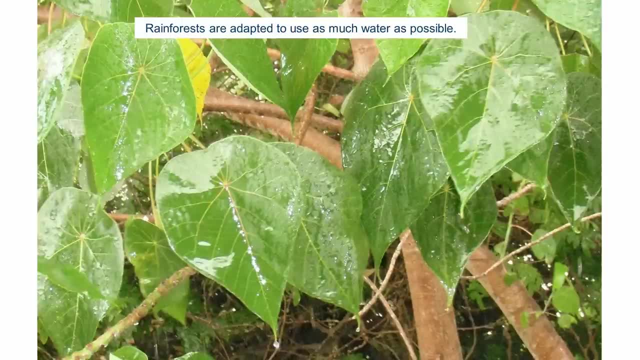 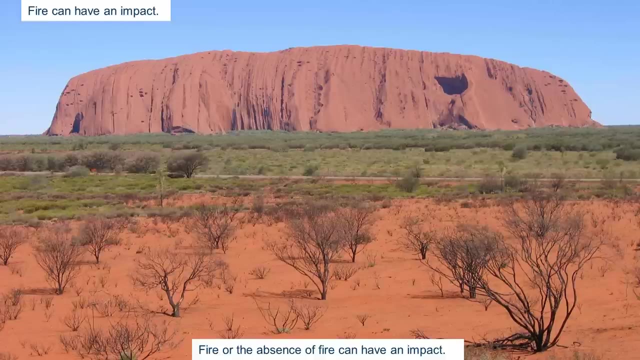 sharp drip tip point on it and that directs the water to the ground. but of course it takes a bit of time for the water to come out of the canopy and down onto the ground. If we have an impact in some areas, of course, where fire occurs, then of course the whole. 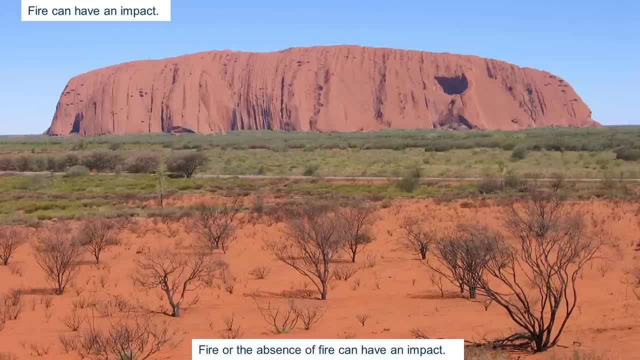 system is changed and so rain in this particular instance would get through to the ground level very quickly in this part of this area, but in other parts of the area it would be very quickly intercepted by the vegetation in that area and, of course, the Uluru rock is. 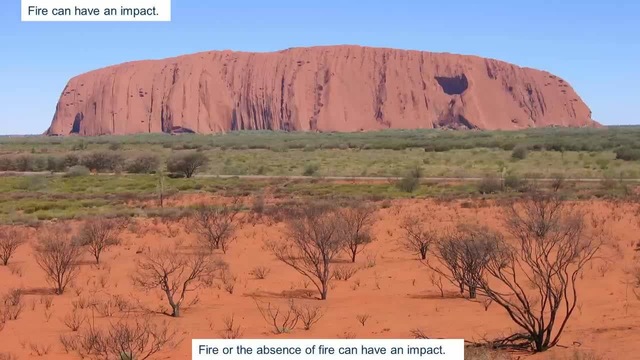 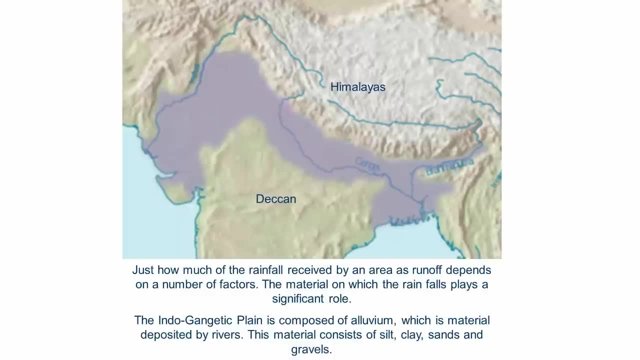 quite an interesting catchment for water too, because the water just pulls off that rock, if you're lucky enough to see it. In the Indian subcontinent again, we've got this very, very large alluvial plain. it's called the Indo-Gangetic Plain. it's made up of the plain of the Indus River and the Ganges River. 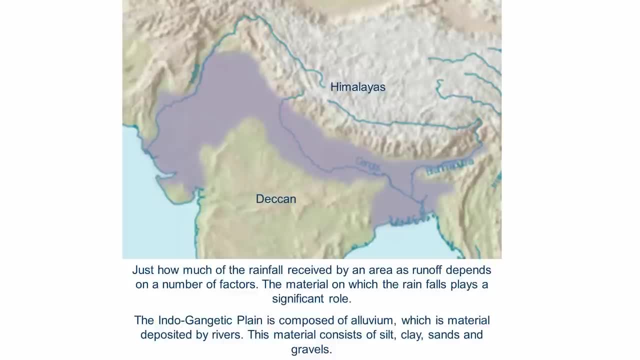 really small rise between those two catchments separating them, and of course the mountains of the Himalayas separate them to the north. but once the water flows out of those mountains it runs into quite a variety of materials that have been deposited by the rivers over a particular time. so silt, clay, sand, gravels will all have an impact on how much water. 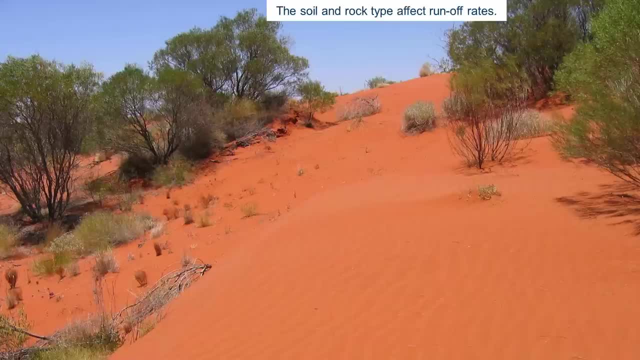 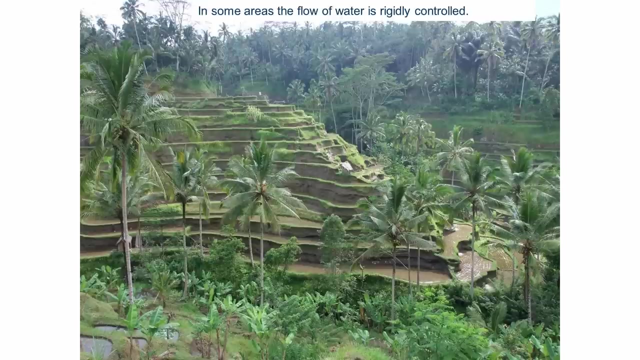 actually makes it through that particular catchment area- Desert areas, sand dunes like this one just near Uluru. The runoff from that is going to be very small, unless there's a very, very, very severe storm. In some areas the flow of the water is very, very rigidly controlled. 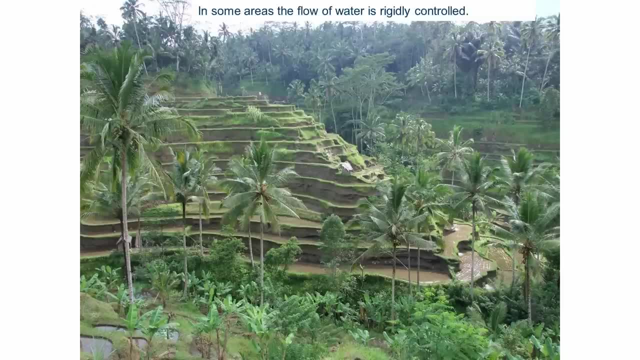 This is, of course, barley, the rice paddies there, and virtually they control the flow of the water down to the last teaspoon. And in this particular situation, again from an engineering perspective, these are relatively complicated systems to model. So what are the challenges? And at times an engineer will need to make decisions to simplify how the system could. 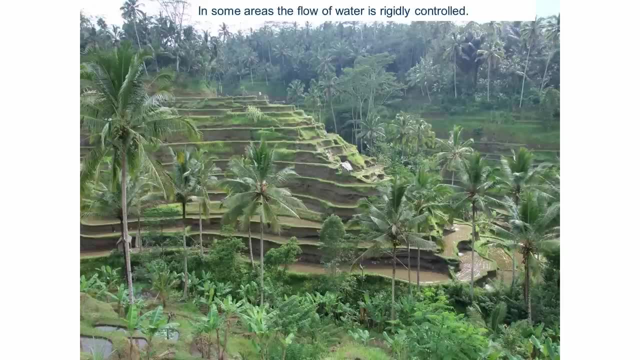 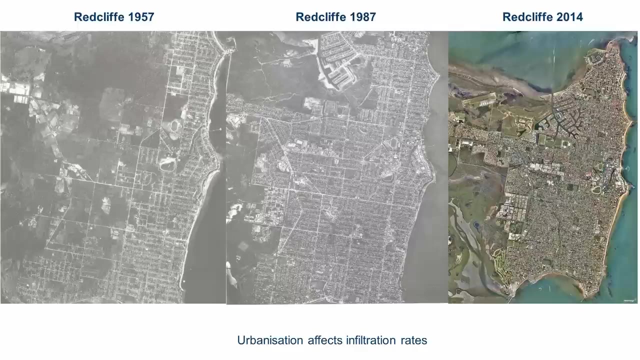 be modelled because again we have these steep contrasts between some of the core parameters, such as catchment slope, as we see, but also depression storage, and again that management of the water in this particular location And moving along this interesting set here just shows how urbanisation affects infiltration. 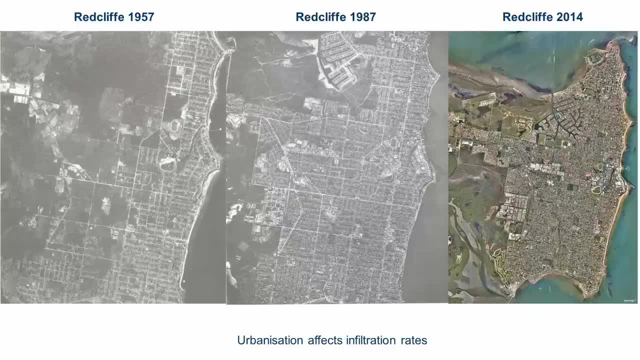 rates. Both Gavin and I come from Redcliffe. Gavin's moved on. I've stayed there, But in 1957 on the left hand side of the screen you can see there was quite a lot of bush. You can see a couple of catchment areas down there on that particular photograph. 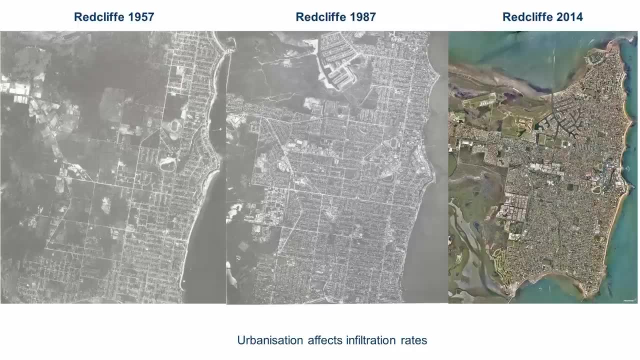 1987. we're starting to get development occurring through the peninsula Quite a lot of vegetation is being replaced, of course, by roofs, car parks, streets, So there's lots of interception, lots of runoff. We get out in one day or two. 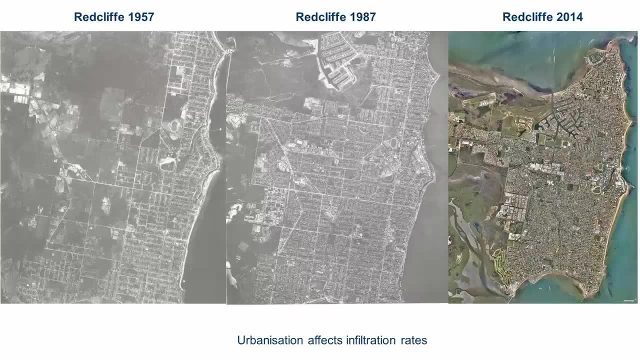 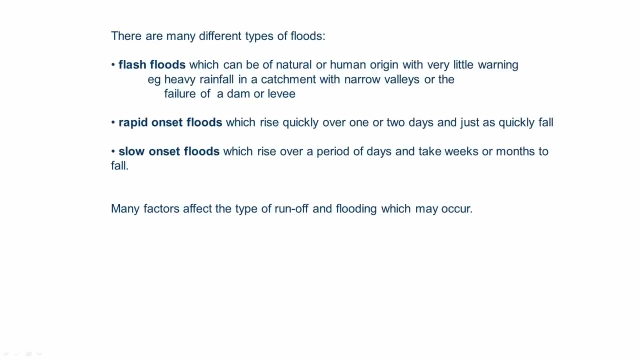 That's the project we're working on to 2014 and virtually there's a nice little green square in the middle of your image there, which is the Redcliffe Botanic Gardens, and most of the rest of the area, unfortunately, has been cleared for urban and industrial development. 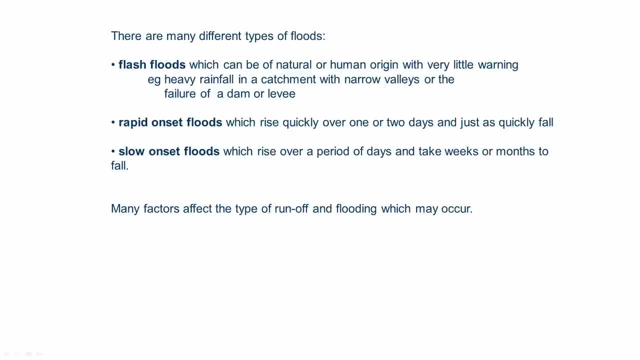 The types of floods that we get: many different types. A very quick one is the flash flooding. It can be natural or human origin. often occurs with little warning. You often hear of campers being trapped and sometimes unfortunately swept away. When we have heavy rainfall in a catchment with very narrow valleys, or we 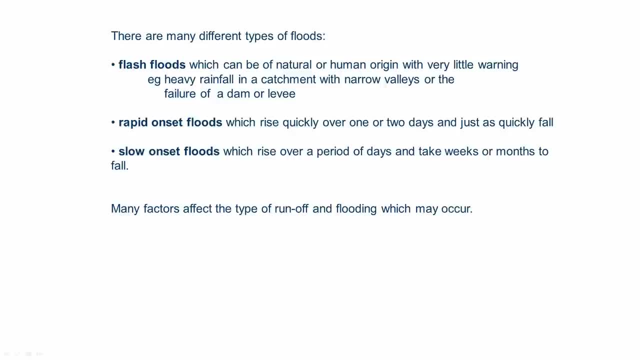 have the failure of a dam or levee in a particular area. Then we've got the other two sorts of floods: the rapid onset flood. It'll rise quickly over a couple of days and fall away just as quickly. Many areas experience this type of flooding. 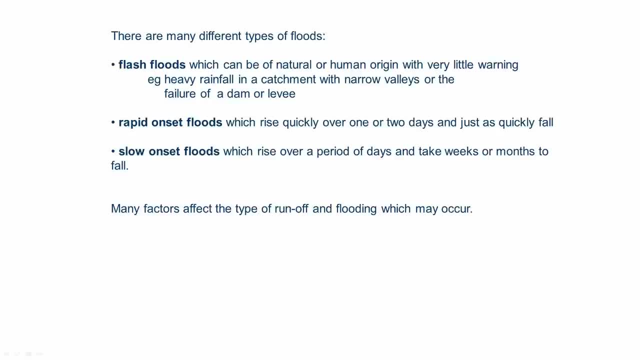 Where we've got low flat areas, like we've got in the western side of the Great Barrier Reef, we've got low flat areas like we've got in the western side of the Great Barrier Reef Dividing range in Australia, We get what are known as slow onset floods. We also 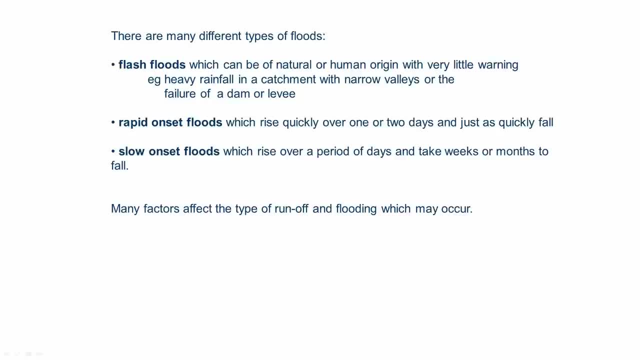 get them in the Indus River too. We saw them a couple years ago- and these rise over a period of days and can take weeks, weeks or months for the flood level to fall. Many factors affect the type of runoff and flooding which can occur in. 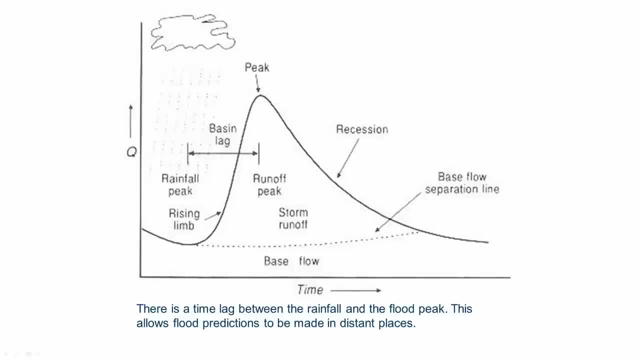 these areas, And just to show it in a graphical form, we get the rainfall, but, as you can see in the diagram here, there's some time lag between when the peak of the rainfall occurs and when the actual main runoff occurs, And there are lots of reasons for this, some of which. 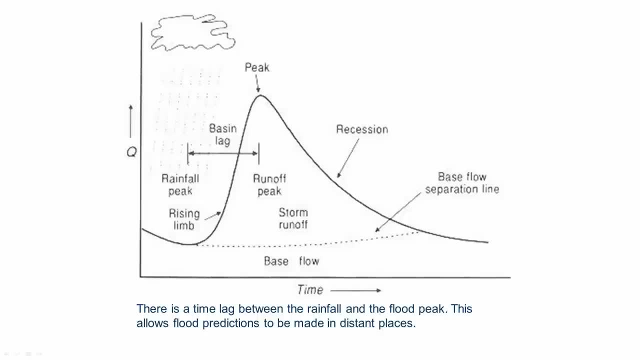 we've just looked at The sort of vegetation cover you've got, the soil and rock type you've got and what sort of agricultural use you've got of the area, And just quickly looking at an example of this. This is one of our rapid onset. 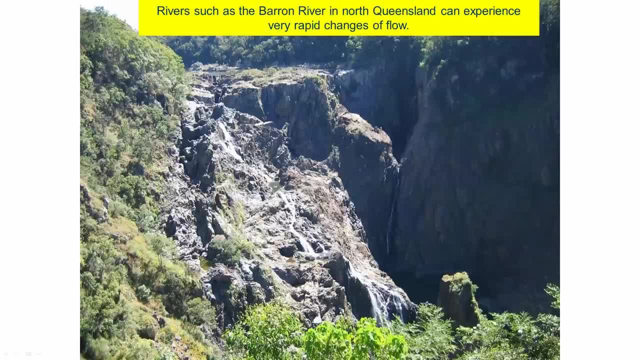 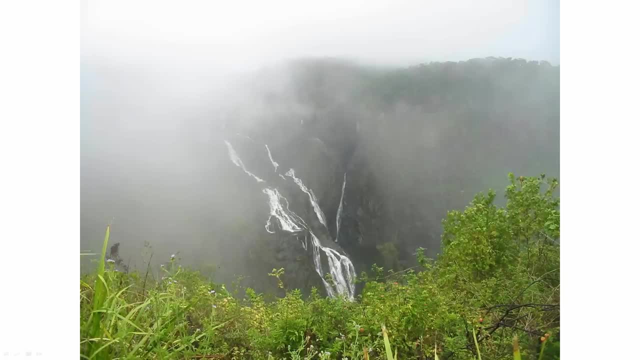 floods here. Barren River made famous for the Barren Falls in North Queensland. Unfortunately, many people will go there and see them looking something like this, But if you're lucky and there's been a bit of rain around, you'll get something where the falls actually become quite major and 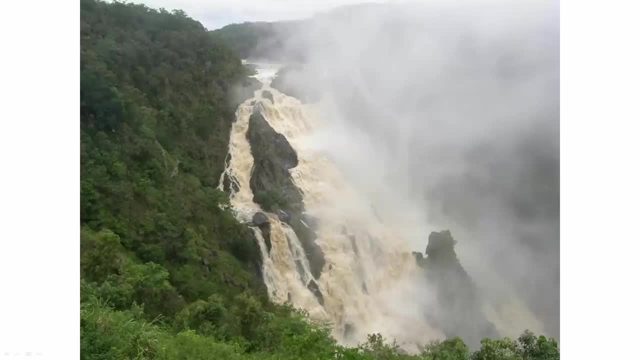 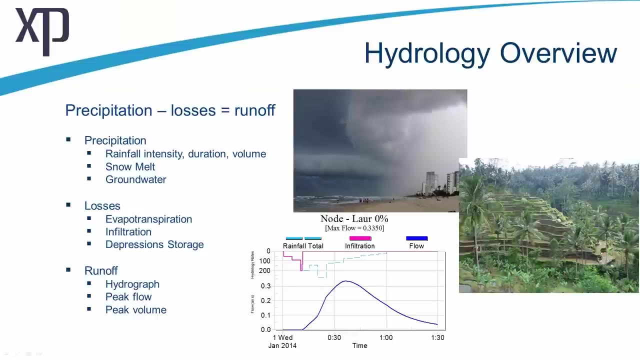 significant and quite spectacular falls, Usually within much quicker than 24 hours, of rain falling in the catchment of that area. And thanks, Dave, That's a great overview of the physical characteristics of the hydrology process that practising engineers have to deal with, And we felt it was a very 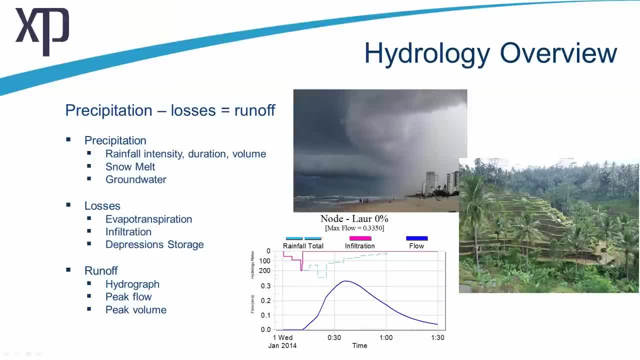 good overview to see it in that sort of format, to take some of the numbers away from general hydrology. Unfortunately, me being the engineer, I might bring some of the technical elements back onto the table And so, just as a quick overview of what David's just described, we 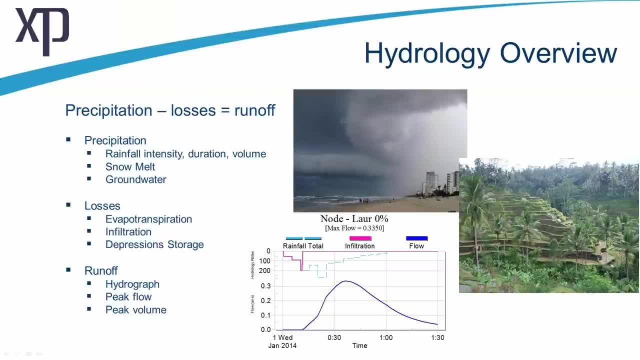 have these functional components. We've had precipitation, that variation between those flash flooding, type characteristics, monsoonal rain patterns, and then we've got the flood patterns, broad area flooding. We have the losses, the evaporation, transpiration, storage, infiltration, And then of course you take those away from each other and we 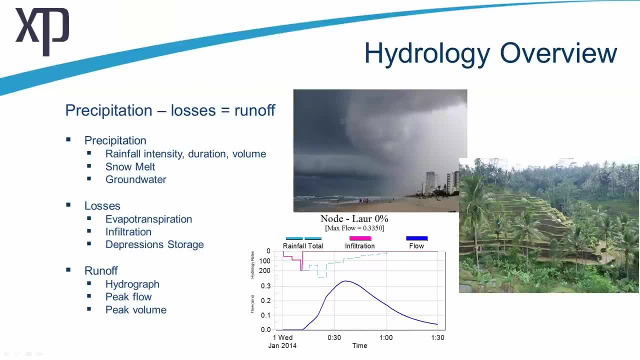 can derive our runoff From a software perspective. the graph in the middle there highlights the variation that you get between: the graph is functionally the storm itself multiplied by rainfall intensity, The magenta line, the infiltration is lost, So we don't have any. 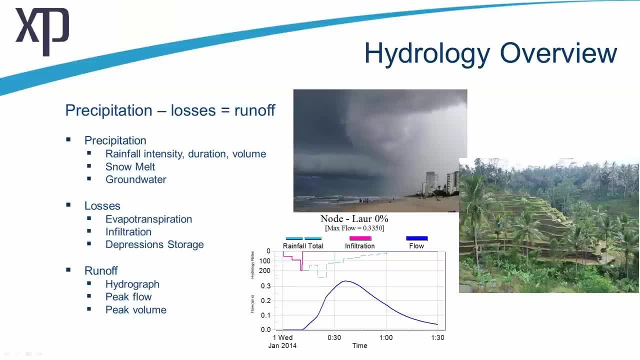 runoff. We can see quite clearly we've lost surface runoff from that component And as the storm continues to build, we get to see the peak. that is actually quite delayed relative to this water. It's actually a small catchment, but we've got about a 15 or 20 minute delay. 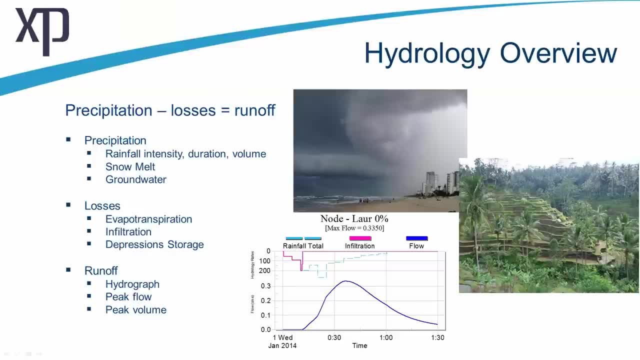 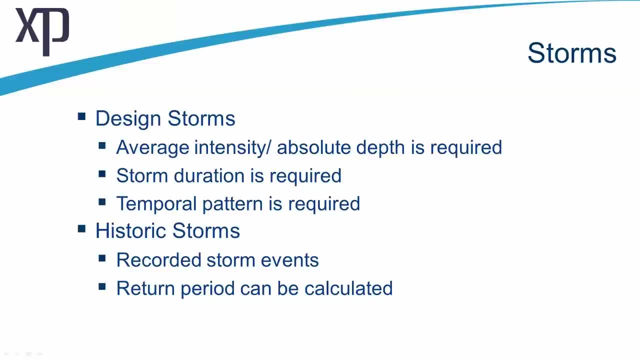 relative to the point at which the peak rainfall itself occurred. on that higher graph From an engineer's perspective, we typically look at two types of storm analysis. We have design storms and historic storms, And that's often a difficult question to try and deal with as to what should a user 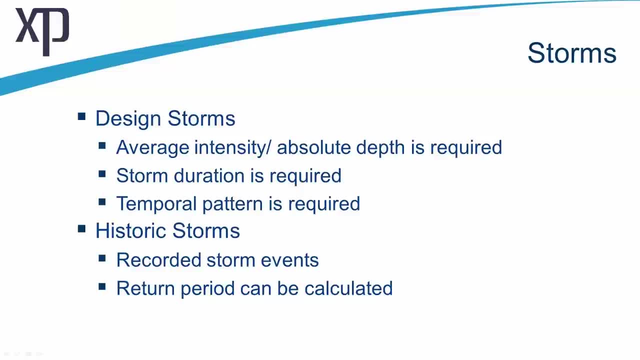 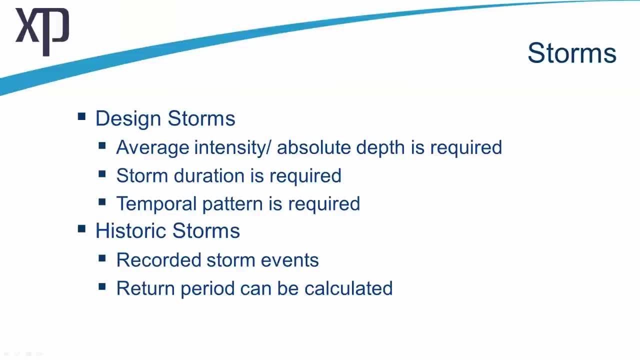 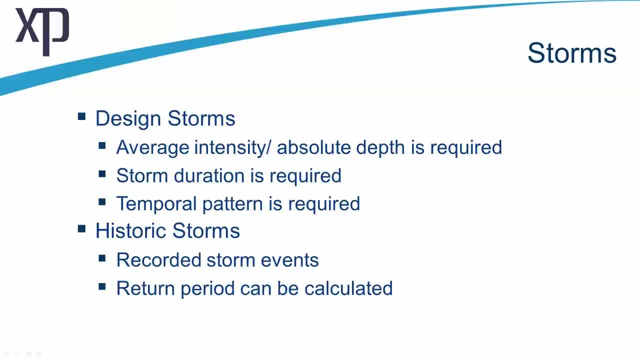 It's nice to meet all of you, So I'm really pleased to be here today, and so we're going to talk a bit about our research information before I go into question 18.. First, we'd like to talk to you again about what we can consider when it comes to 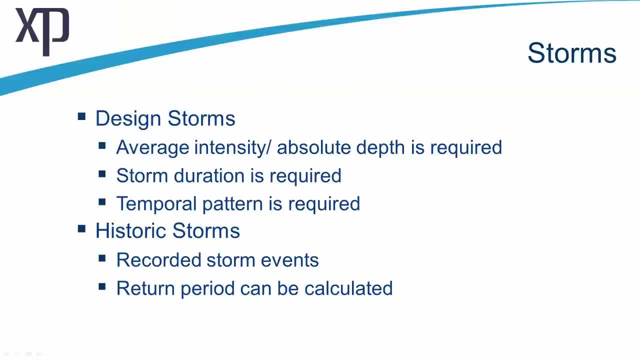 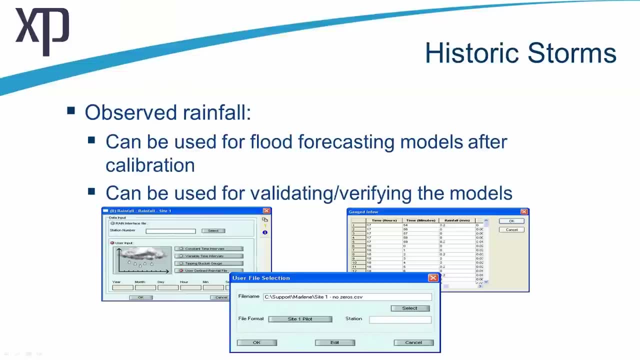 additional cooldown trends toward the long-term we could expect to see in the near-term datac Palestinian sea, 따�ed. So, as I said, all of those things matter as the result of our research. Historic storms are typically obviously that function of observed rainfall, but are used. 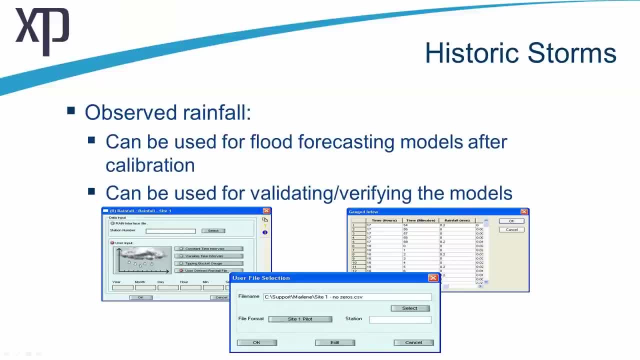 to identify how major catchments in particular perform, and particularly important if you are looking at trying to calibrate a numerical model against a real world situation. For example, the Brisbane River catchment at the moment is going through a big update to its analysis pursuant to the major flooding that was in this particular part of South. 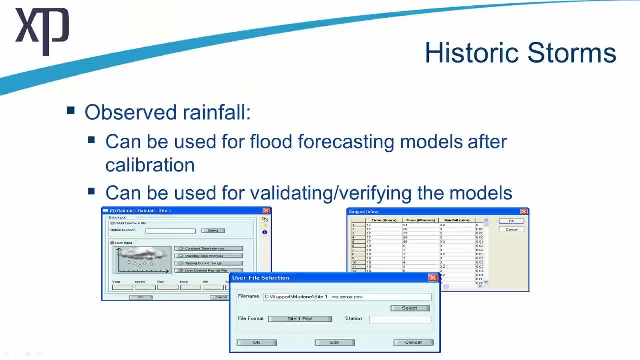 East Queensland and the broader Queensland area in 2011, and, of course, the key part of that is to try and validate that information and also provide our Bureau of Meteorology with improved data to forecast the impacts of flooding in terms of providing flood risk warnings to the community. 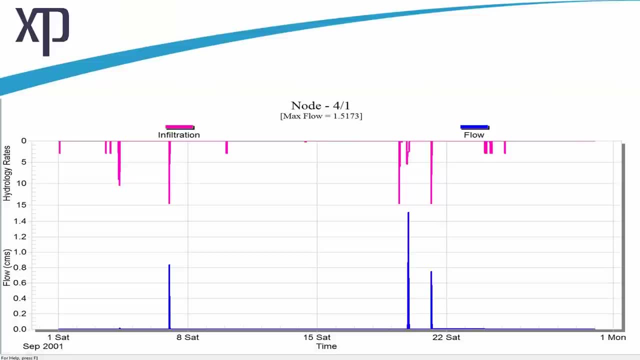 This is just a simple graph which sort of shows how, over the course of a rainfall event, that infiltration can actually be quite a dominant problem. So we've got flow as the blue line at the base and you can quite easily see that we've actually lost these components of this particular catchment, which is a rural catchment, and we 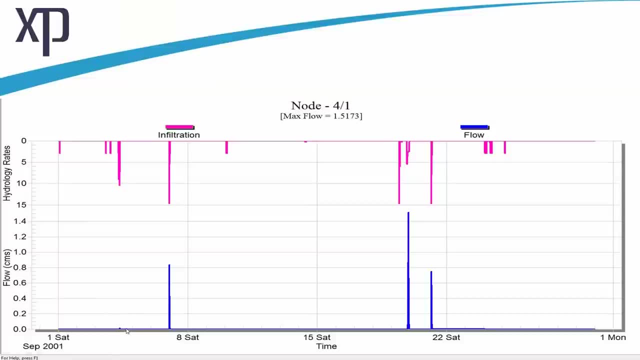 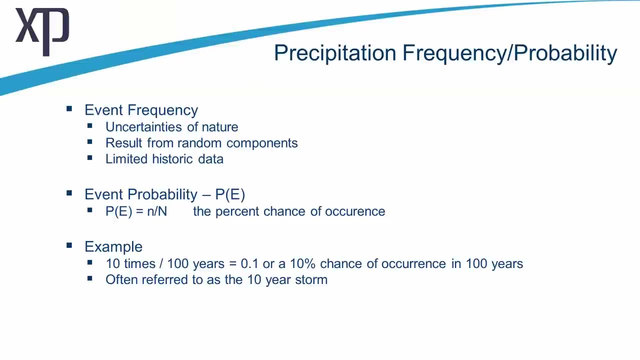 only have these tiny blips in rainfall in runoff. I beg your pardon, But models can quite easily assess this. again, it's getting the information. to compare it against it makes this type of analysis difficult From an engineer's perspective. again, we need to understand some of the statistics. 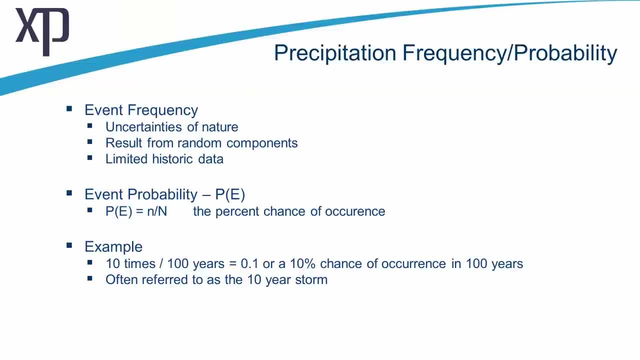 behind what we're trying to analyse and that makes us look at event frequency, the probability of said events, and trying to get a generalised relationship between the two. A standard example is what the newspapers like latching onto will be a statement that any particular storm may be a one in ten year event or a one in a hundred year event. 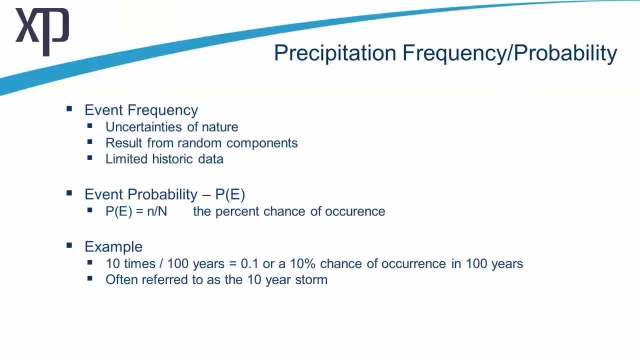 So that's a standard example. But what does that really mean? and so, functionally, if we look back at our historic records, if a given rainfall occurs ten times over the previous hundred years, if you have a hundred years of record, well then we might generalise that statement to say that well, it's a point. 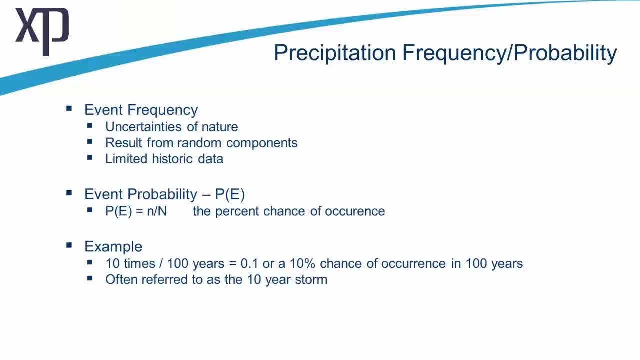 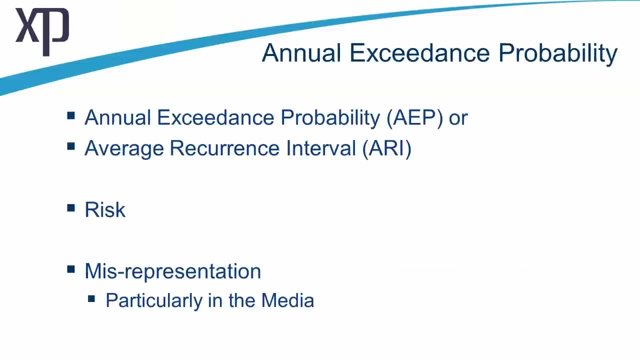 one storm or a ten percent storm or that one in ten year storm. Functionally those statements all hold true, but again it does lead to the potential for misrepresentation, Particularly in the middle. Some areas are moving away from talking about the one in so many years relationship annual. 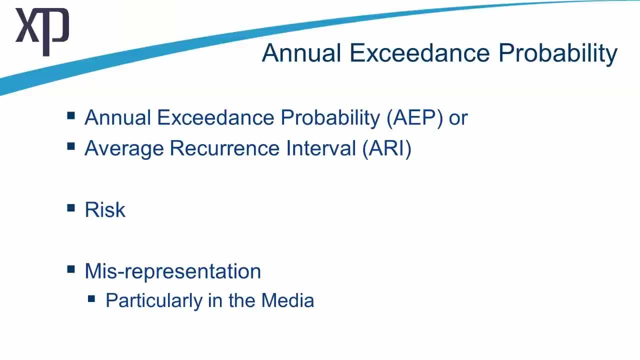 exceedance probability option. but again, that's not widespread, although it's certainly happening in Australia. Because the big thing is, if people say I've had this so called one in a hundred year storm, there's clearly a risk that is implied against that particular rainfall event and as engineers, 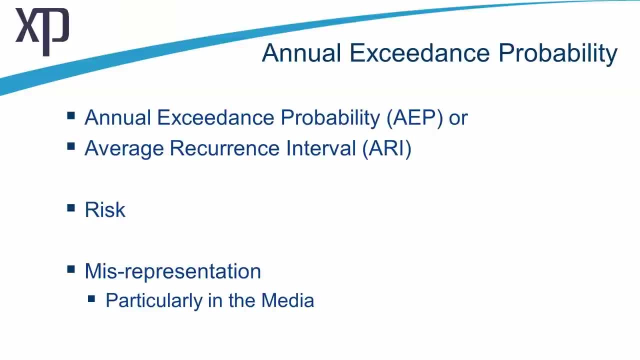 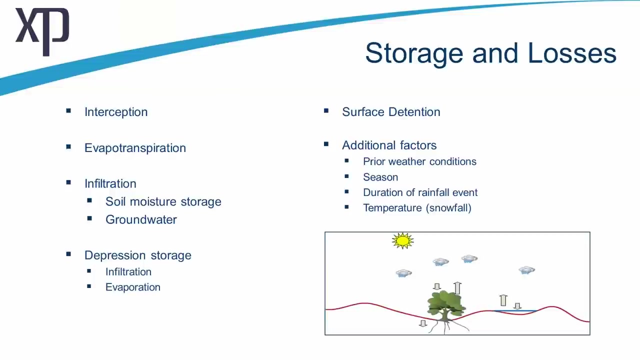 we're typically risk averse. We want to make sure that we're providing the community with the best potential engineered solutions from planning perspectives and look at being able to provide mitigation options in response to these sorts of storms. Just a quick summary. I won't go through this one in a lot of detail. 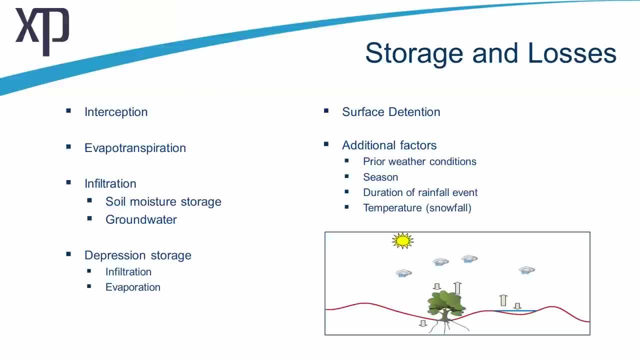 David's done a great job talking about this generally, But these are the core parameters For the one in a hundred year storm, the best potential for mitigation. I'm not going to go through this one in a lot of detail But as you go along and over this years, plan policies from storage and loss perspectives. 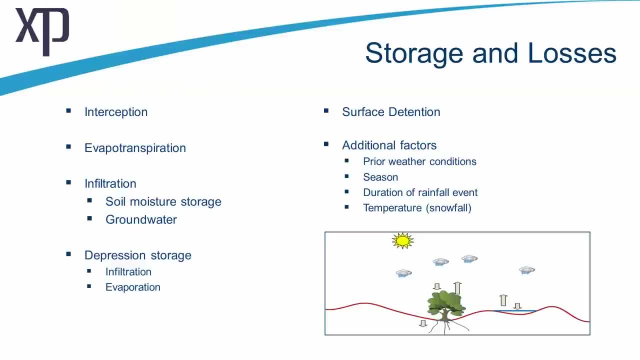 where, again, relative to our inflows and pursuant to our inflows, and losses do occur and losses are not in that way subject directly to the storm itself. Again, we will have these long duration runoff events that exist beyond the grade dividing range here in Australia, where there are a lot of places and towns along the way along. 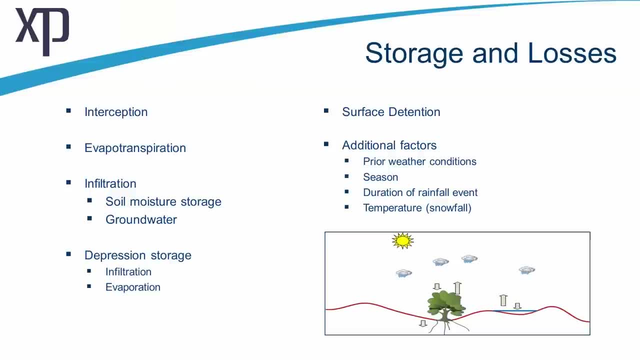 the Murray–Darling system, but will typically have what's called as sunny days. Essex is a tradesman island. floods. The rainfall may have occurred two weeks prior to the event and they can be having a great day when the flood turns up. So these losses are definitely a continuing element. 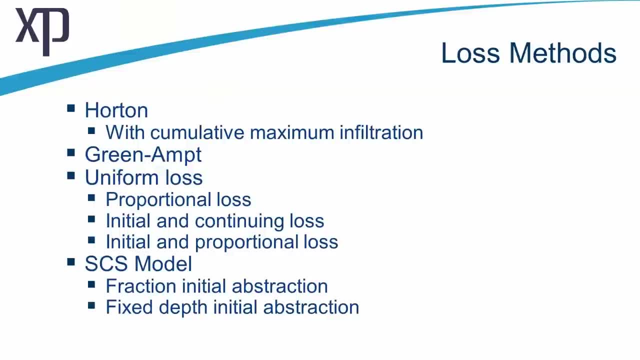 relative to our rainfall From a modelling perspective. in a lot of software packages we have these typically standard loss methods that are available to us. I won't go into these in a lot of detail today. it's definitely a 101 type discussion. didn't want. 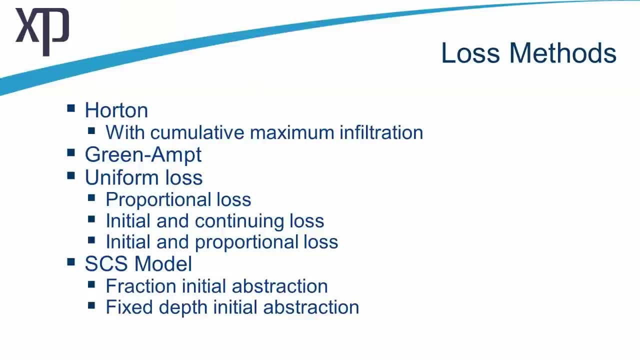 to bore people with the calculations on this particular front, But the core ones being Horton, which is an initial and asymptotic decline method- don't stress too much about those lovely terms- but where we start with a high initial infiltration and that then weans its way down to that ongoing infiltration rate which, depending on the catchment characteristics, 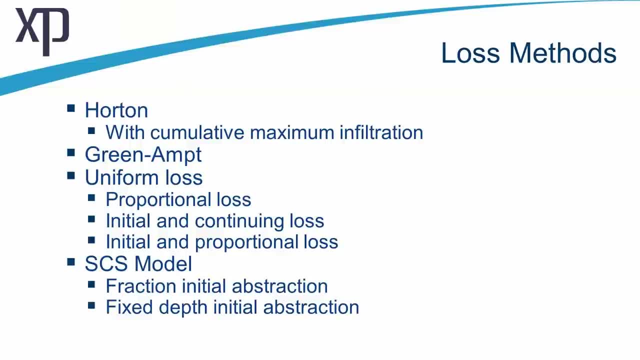 maybe is going to be a little bit higher than that. So we're going to be looking at that as low as 1 or 2 mm per hour ongoing, and that's the kind of information that's definitely important in those long duration, sunny day type flooding situations. So Horton's method. 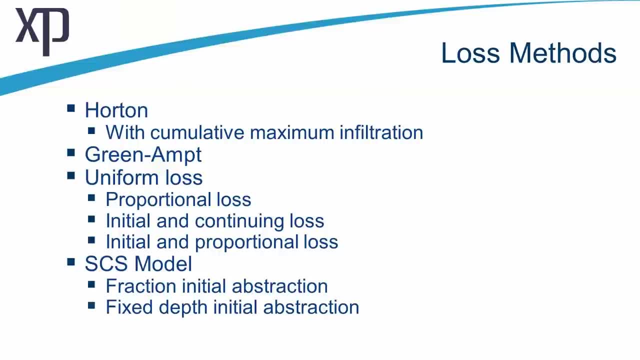 is definitely a loss method that can be used as a continuing loss method, The common one in Australia. I'll sort of skip over GreenEv. GreenEv is used definitely in the United States and other key parts of the world, But the main one that design engineers that use design. 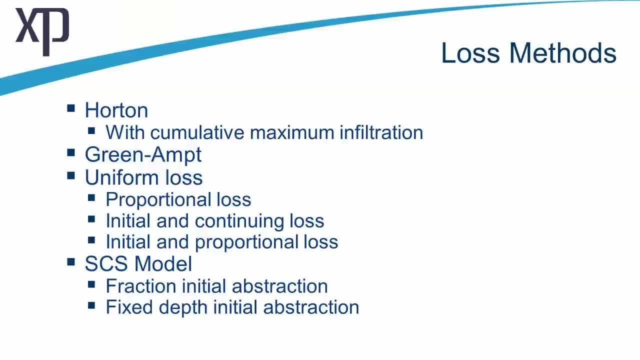 storms apply will be the uniform loss method, Whether they be in proportional losses, where a proportion of the storm itself at any given time frame is lost, or initial and continuing losses, where you can have a burst component and then an ongoing hourly rate loss, or again initial and proportional loss, The SCS model. 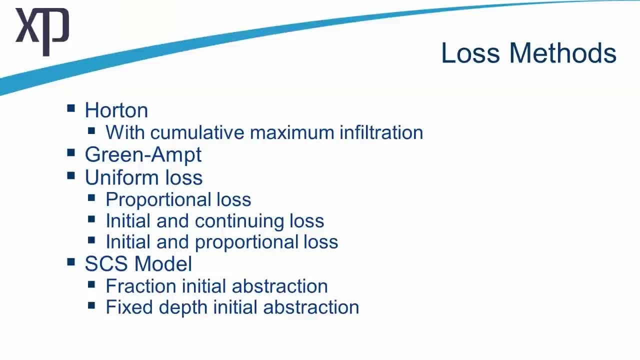 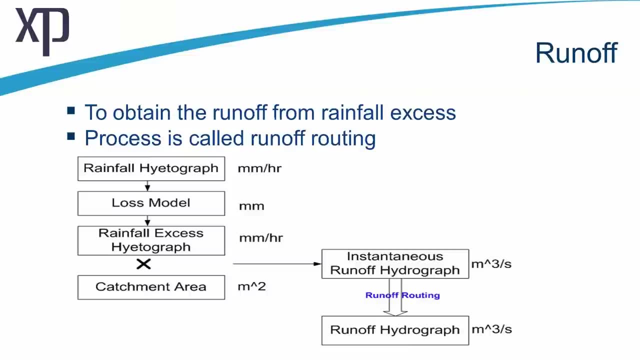 is the soil conservation service model where again, it's similar to an initial loss, but a fraction of the initial loss abstraction pursuant to that point. So the SCS model is similar to that point. Again, this is sort of a modellers overview where we need to apply. 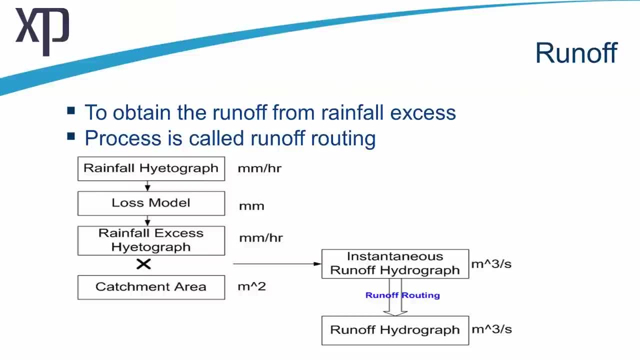 our rainfall, subtract our loss model, identify the excess hiatograph which we sort of showed on a slide previously, multiply that by the catchment area and from that we'll be able to derive an instantaneous runoff rate When we calculate that out over a long storm event. 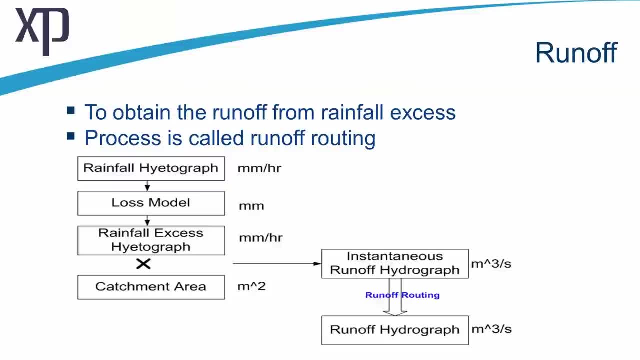 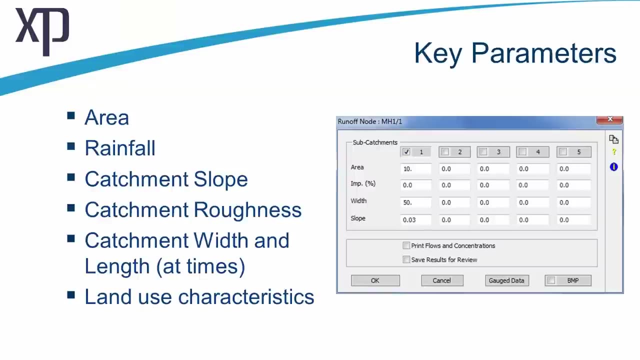 or a design storm event, we'll get a dynamic hydrograph. We can route that calculation through a storage model and then we'll determine our final runoff hydrograph. Some of the key parameters that a modeller needs to take into account, of course, are dominated by the catchment area itself. Rainfall is important, whether that be in intensities. 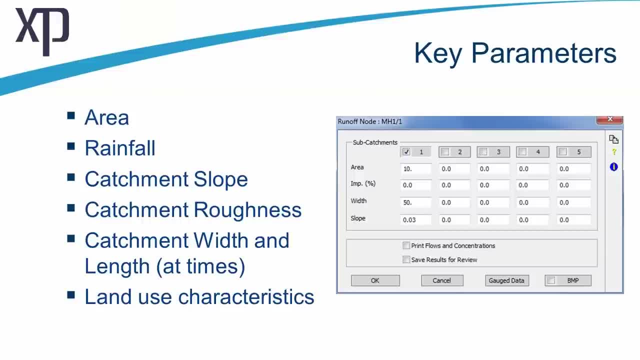 or rainfall depths, depending on how you apply it to the software. You can also determine how much rainfall you need to take into account. You can also determine how much you need to take into account. A catchment slope does change the performance of response times. 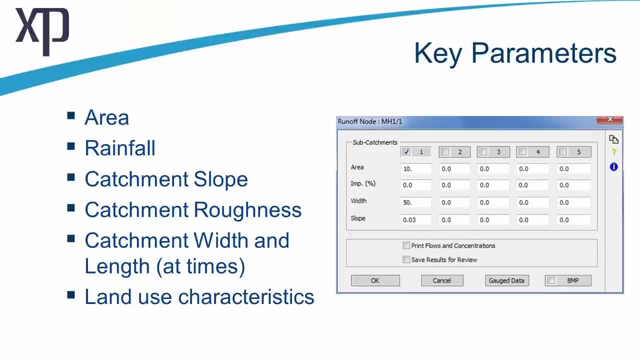 Catchment roughness. where David showed us the great shot up north was the variance with the forest and the road environment And some particular methods to apply catchment width and length to their calculation sets. And finally, the land use characteristics may also affect the loss. For example, a carpark would have obviously a very low annual yield, but 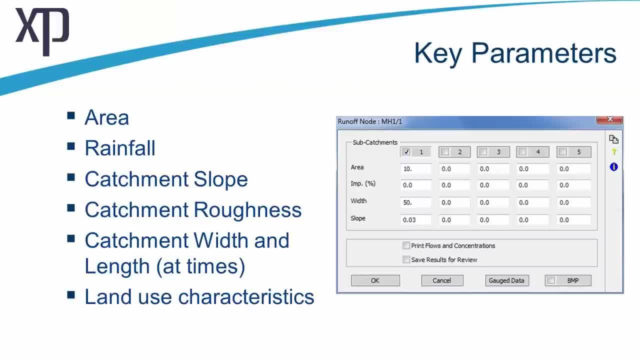 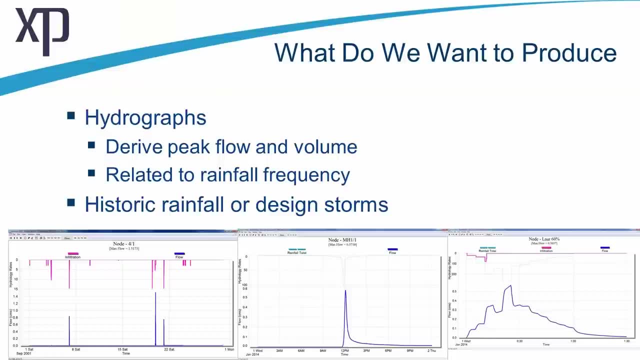 initial loss or continuing loss again versus that forested or undeveloped environment. And so what do we want to produce when we undertake a hydrology study- And obviously hydrographs are the key output where we're trying to derive peak flows and volumes. These 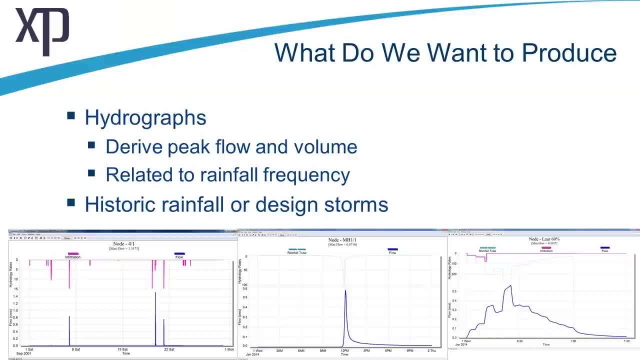 results are functionally related to that rainfall frequency. and in this few slides I've shown the sort of variation between a continuous simulation shot- we saw that a couple of slides ago. it's the same shot- to a very intense soil conservation service hydrograph, which 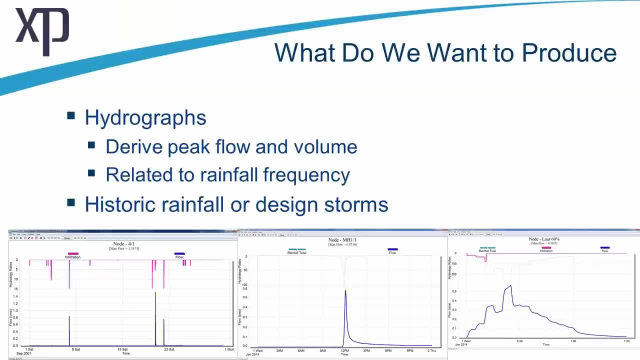 is a centrally weighted 24 hour storm And that particular storm is actually used in New Zealand, Korea, parts of Japan and Canada, as well as widely across the US. So it's not commonly used in Australia but can be at times. And on the right hand side we have an Australian temporal pattern: 60 minute 100 year storm. 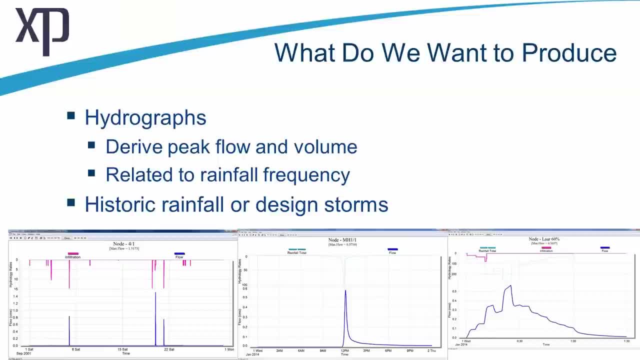 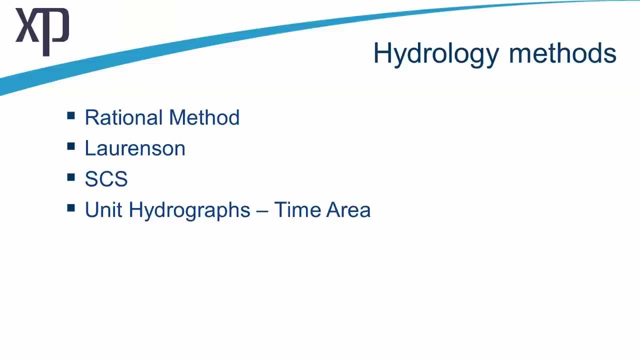 And essentially the analysis of this information is really the hard part From a routing perspective. we have a number of hydrology methods available to ourselves within the engineering fraternity. The most basic of these, or the simplified method, is definitely the rational method, And then we have some more dynamic hydrology methods. 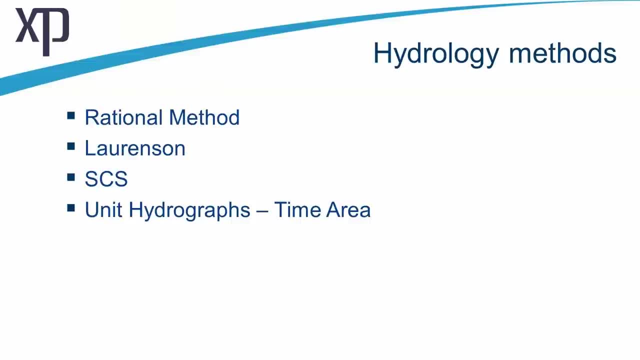 In the form of Lawrenson's method that may also be referred to as the rafts method. One thing I do note that rafts, which you can utilise in XP rafts, is actually stands for the runoff and flow training simulation, So in and of itself is not actually a model. The SCS methods. 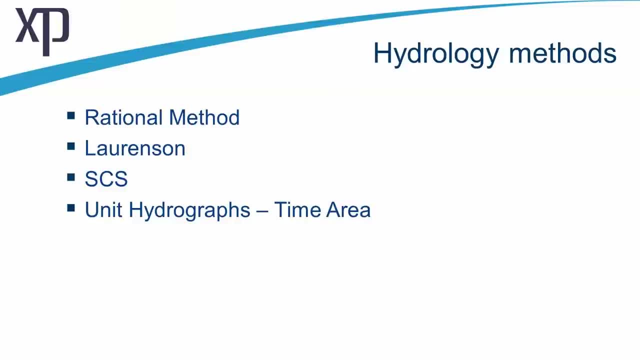 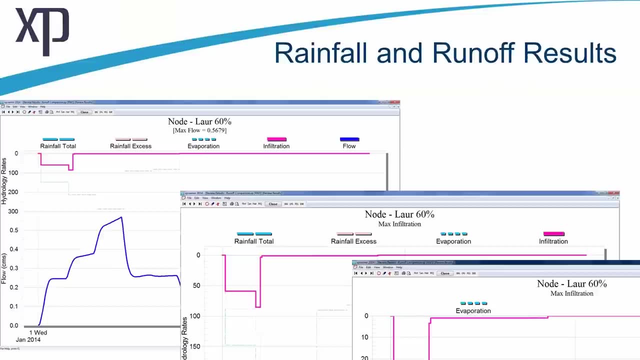 are soil conservation service methods, and unit hydrograph methods such as the time area method are available. Unfortunately, this is not prepared for the next slide. I've shown quite well on my power point but we get to see the variation. we have The overall view that you are getting the results set to the left, showing the full storm. We 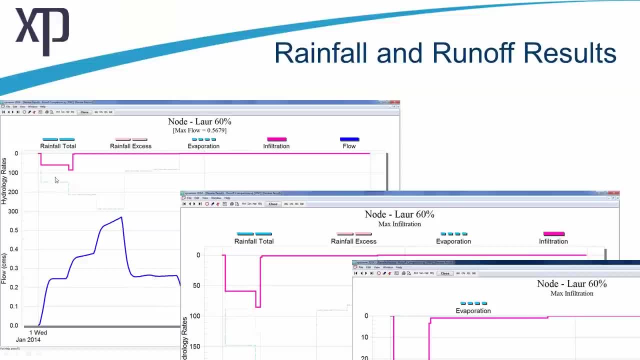 have the raft at the lower component of this graph versus the total rainfall which is the blue dashed line. It's a sort of mimic of the actual big part. you can see the rainfall excess relative to the infiltration Evaporation is right at the top. it's quite low in this particular model For this particular. 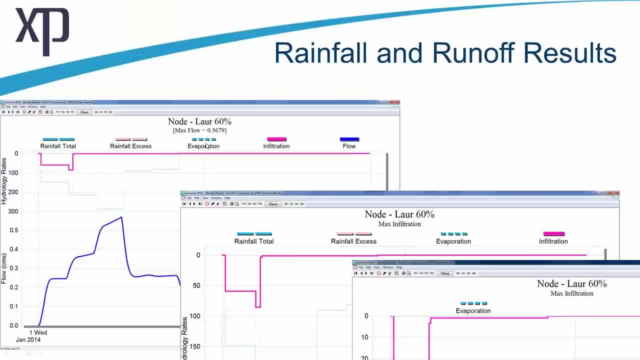 graph. it's only showing about an hour and a half of time and you might expect on any given day, even in a relatively arid area, infiltration and evaporation rates in the order of 5 to 10 mm per day on a particularly dry day, and of course you don't necessarily. 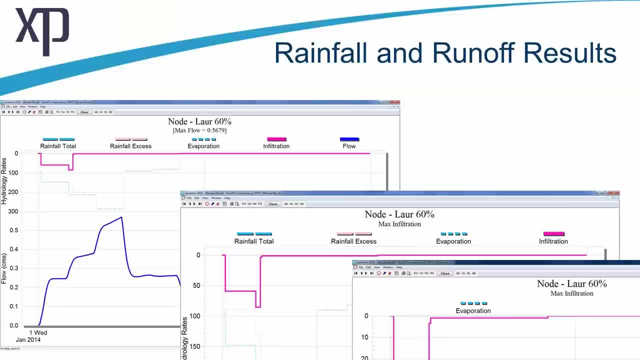 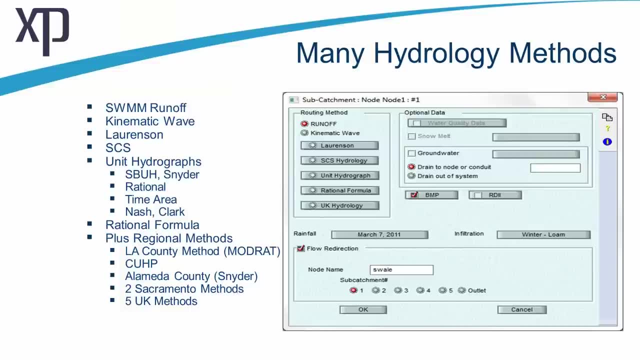 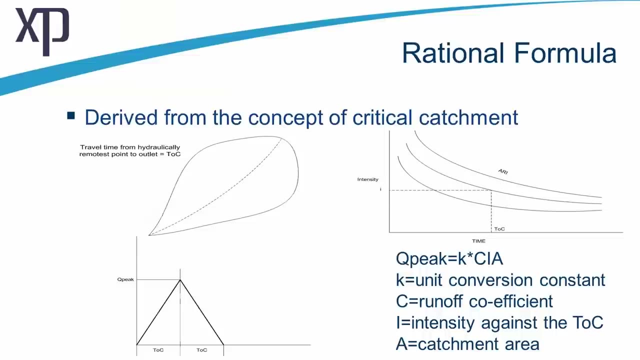 expect particularly dry days prior to or after a rainfall event. From our software in XP-SWMM, there are a number of hydrology methods that are available to engineers for application. The rational method, again, is the simplest of these, which is derived from this term: 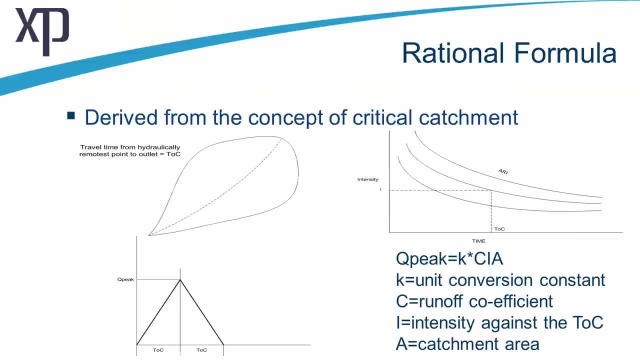 of identifying the time of concentration and from that you are deriving the critical storm. It's very much a simplified method. We have simplified it. There are coefficients to basically incorporate your losses relative to the tidal catchment area. The intensities are derived based on this time of concentration. 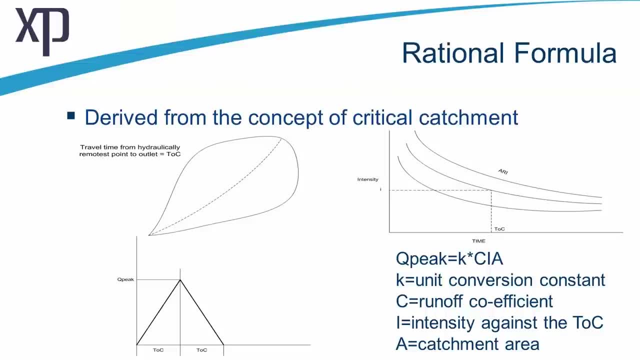 You look at an intensity frequency duration table. If, for example, you had a 15 or a 25 minute time of concentration storm, you would expect a relatively high intensity compared to a long duration storm that may cover in excess of 20 minutes. If you had a long duration storm, you would expect a long duration storm that may cover. 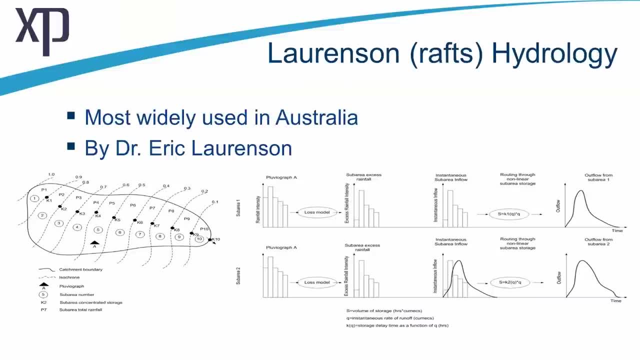 in excess of 24 or even as high as 72 hours. from a design perspective, Lawrenson's method or the RAFS hydrology is definitely widely used in Australia, but it is also used in parts of the Asian areas, China, etc. 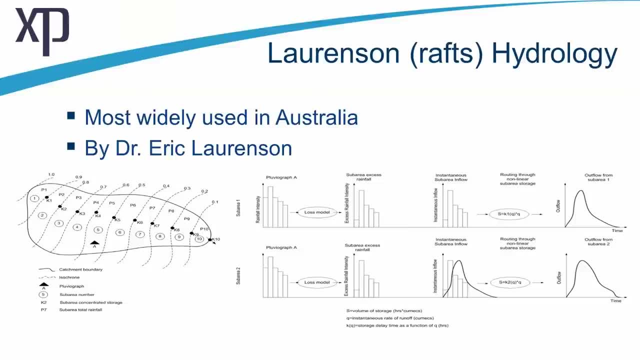 And what this particular method does. it takes your total area and it takes an additional calculation to subdivide any given sub-catchment into 10 equal areas. It routes those through each other using a storage equation And the result of that is a dynamic hydrograph. 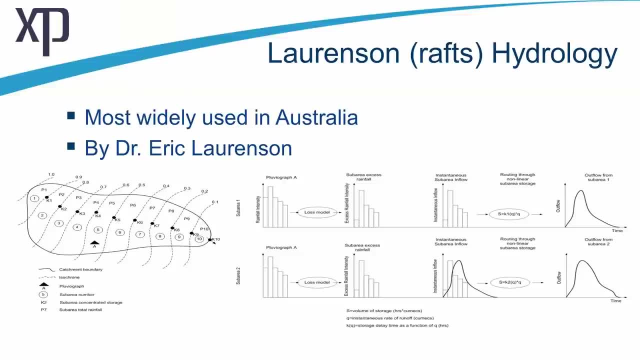 And it's a well-known and well-reported method And if people are interested in more information, they can obviously contact us to find out more about this method. But it is also detailed in the Australian Rainfall and Runoff documentation as well. That's just a quick summary. 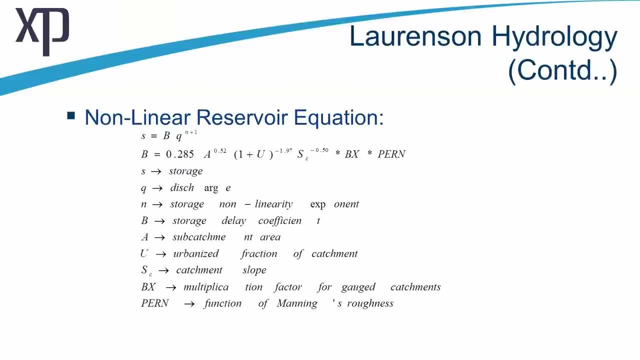 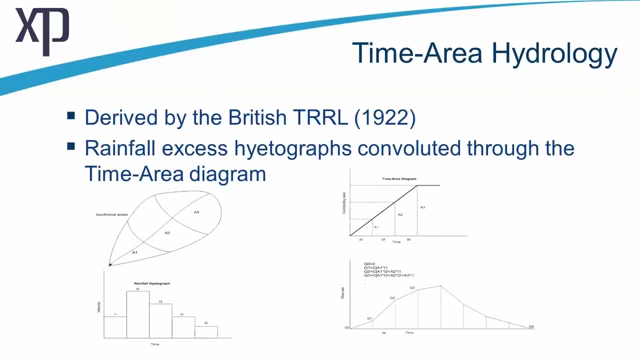 Again, I didn't want to go into too much maths in this presentation. Sorry, But that is the core equation and the parameters there, and by all means come back to the slides which will be available for download after this webinar. The time area method is derived in England and it is functionally a modified rational. 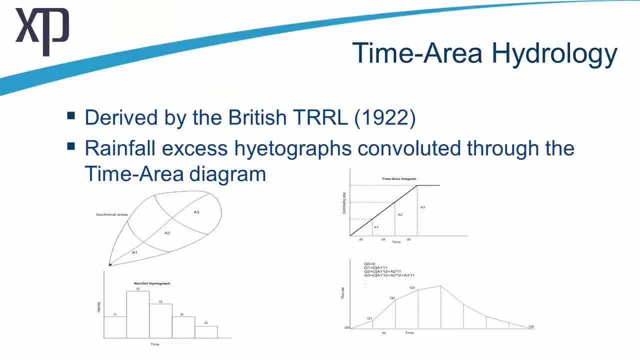 method. That's probably the simplest way to describe it for those who may or may not have struck this particular method, But we do get to utilise variable data. We get to use variable rainfall components instead of having a static storm, And again, that's the kind of output we see on the bottom right-hand corner relative to 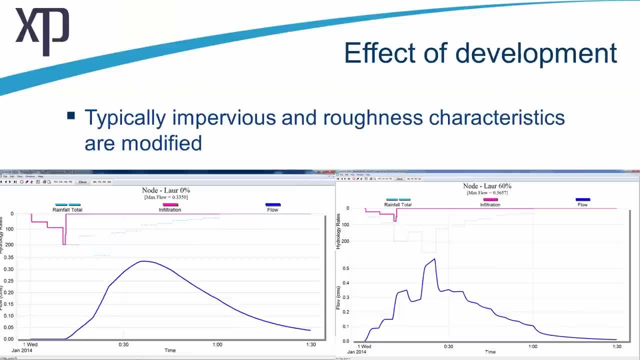 the catchment area top left. Now, development is one of the key things that engineers do want to assess, which is that change between the impervious characteristics mainly, and when we change the impervious characteristics, we inherently change the rainfall. 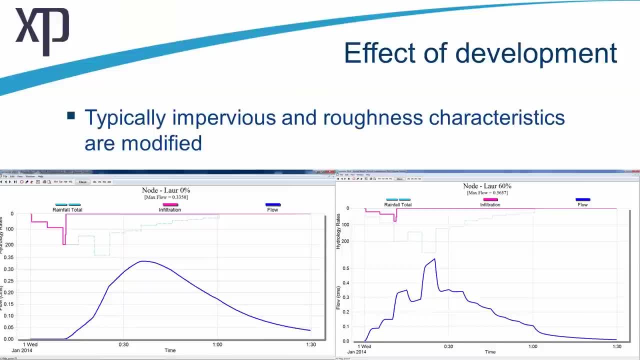 That's what we want to do, So we want to be able to test the values between the threat and the external conditions, so that we can get an idea of what the problem is, where the risk factors are or what the potential risk factors are. 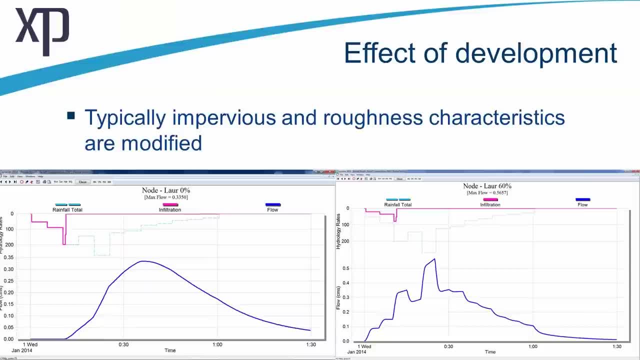 So, as we get into this part of the analysis, we'll show you the difference between the don't sound like large numbers if you were to extrapolate this catchment out, which is only covering, I think, a single hectare. as all, this particular model was a simple model. 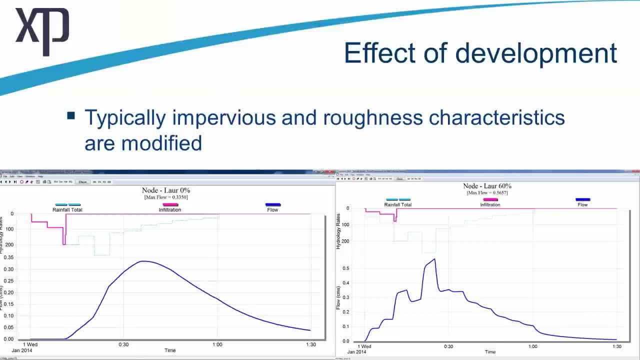 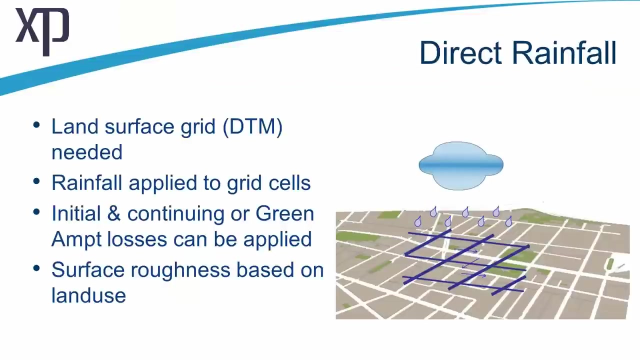 we set up, extrapolate that out to regional catchment. wide changes and urbanisation has significant impacts on our natural systems And of course you may wish to, from a hydraulic perspective, look to resolve that with engineered solutions. Just before we wrap up the latest, I suppose, advancement to hydrology that is now available. 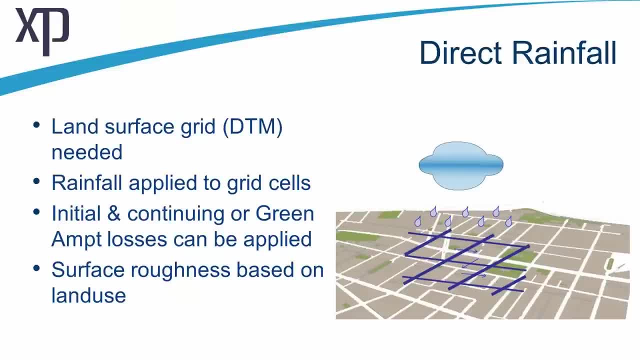 to the engineering fraternity is direct rainfall or 2D rainfall, And it is being seen as a simplified method. I, in part, will say that it is taking the engineer away from hydrology at the moment. I will say that the most difficult thing to define is the first point that David discussed. 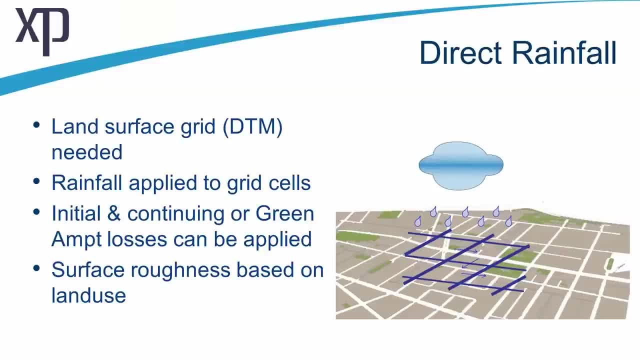 earlier, which is the identification of those major catchment boundaries. Once you have defined your major catchment boundary, you can apply a polygon using a GIS method and apply rainfall directly over your catchment to a digital terrain model and apply losses based on land use. 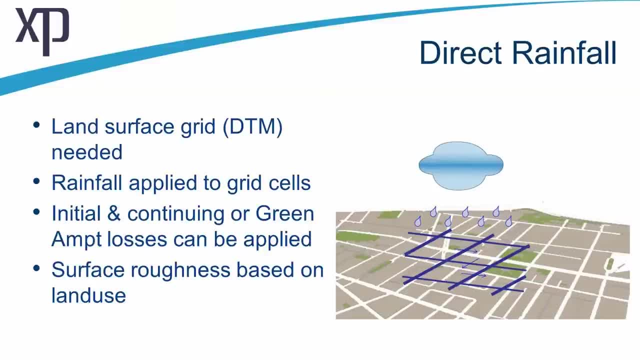 It is very highly exploitative to use GIS methods to identify potential rain coverages for particular areas. Once we have made the decision to only use a GIS method, we have to think about the local structure and the other impacts that we might be facing with that. 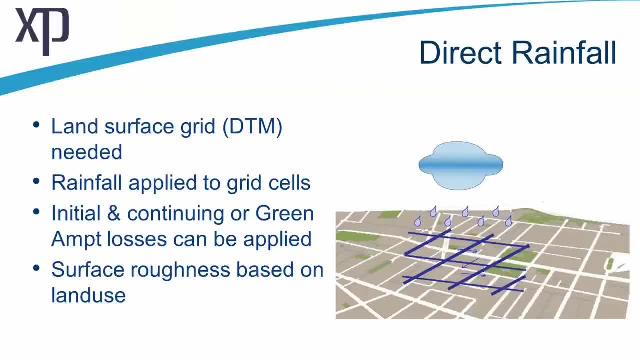 Now, as I mentioned earlier, the kind of type of data that we use to consider changes to our new system would be the location and the area. We have been doing this for a long time. We will try to do the current implications as we move forward, but rather than simply. 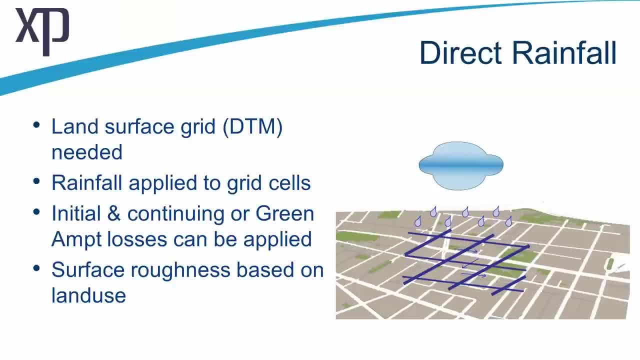 going back and forth. we think that is the most important thing that we need to do. inaudible example: where we have those rapid changes of storage in the rice paddy situation. That's not saying that 2D models particularly love doing those kind of steep slopes, but it could. 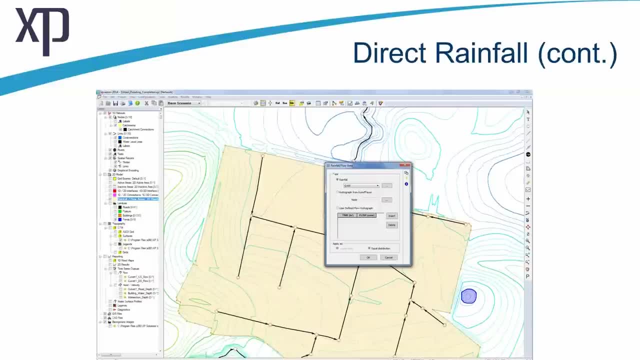 be done From inside the model. from a modelling perspective, you do need to have good data. The most difficult data to come by is typically the terrain itself and thankfully, with advances in aerial data capture and aerial photography and LiDAR techniques, we can quickly apply that information. 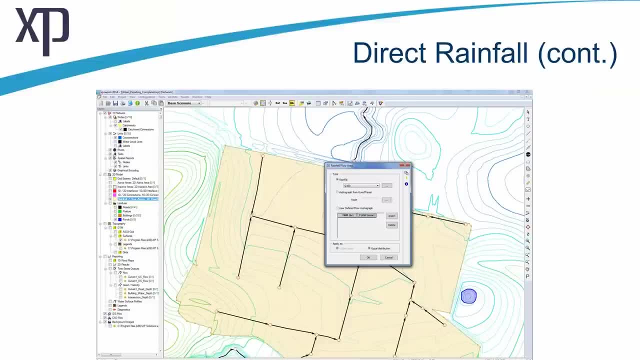 if it is available in your area. We can see here. I have just drawn a simple polygon over an area, and where this orange shaded polygon sits is the area that I am going to say rainfall will occur to assess the performance of what, in this particular example, is actually a minor. 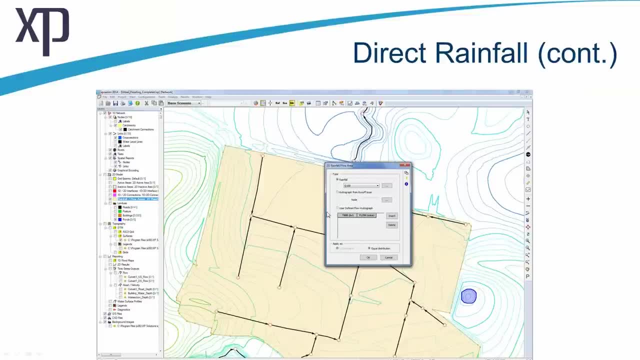 drainage or pipe network system From a dialogue box. we just simply need to say this is the rainfall. I wish to occur in this zone, and I would also define other elements such as buildings, road, land use characteristics, and then analyse the performance at the creek. 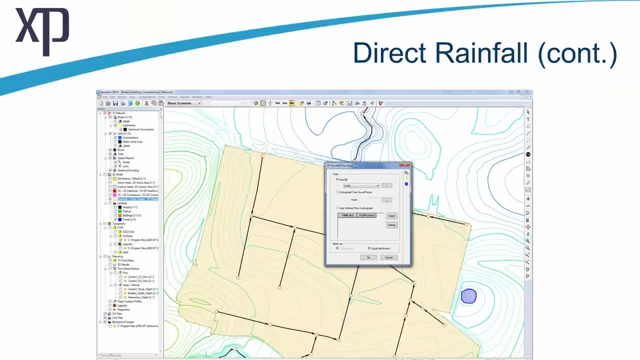 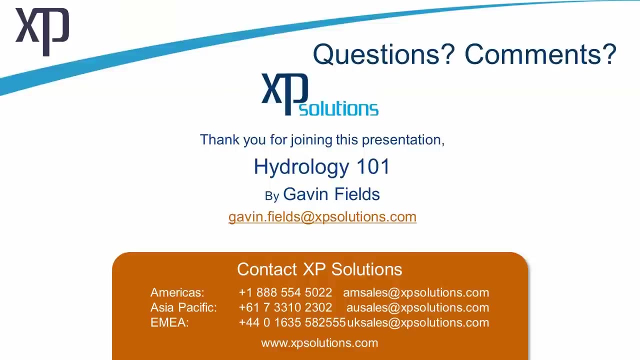 at the northern end of this site. So that's sort of the more recent change to hydrology. That's the end of our session today. Hopefully that wasn't too stressful a session. We wanted to keep this nice and simple, to talk about those physical characteristics. 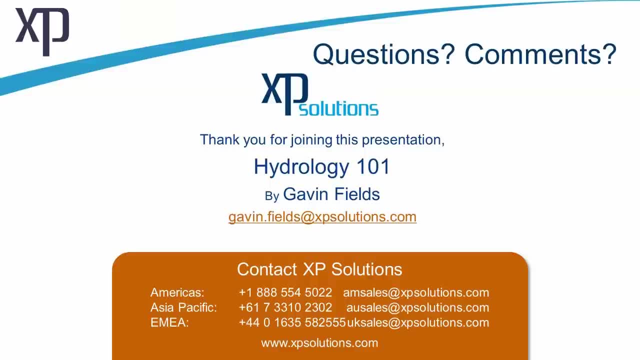 And also some of the methods that are available to engineers and designers, and we really do welcome any questions If you haven't been asking them in the background. I have certainly heard my colleagues typing away busily in the background. If there is anything in particular, 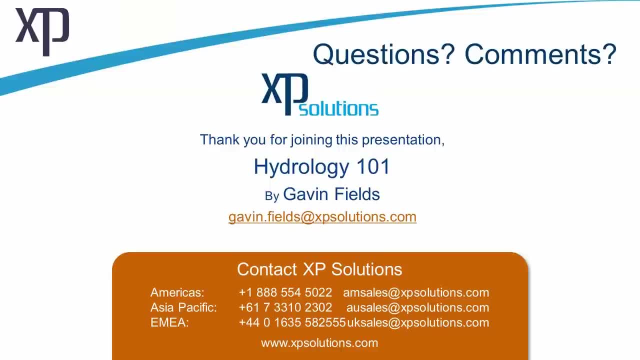 you think of pursuant to this session, by all means contact us on the details at the bottom- there, Obviously, we are the Asia Pacific Zone- or via our email address, which is au sales at xb solutions. Thank you very much for your time today and thank you, David.